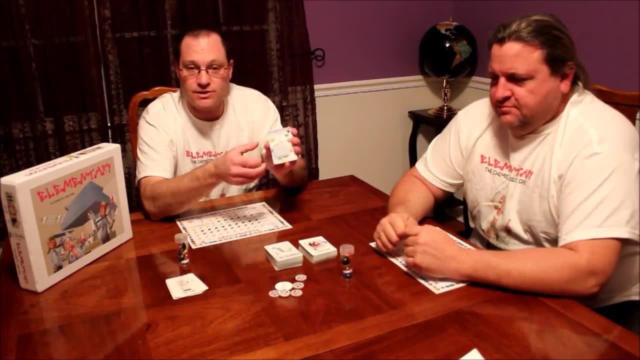 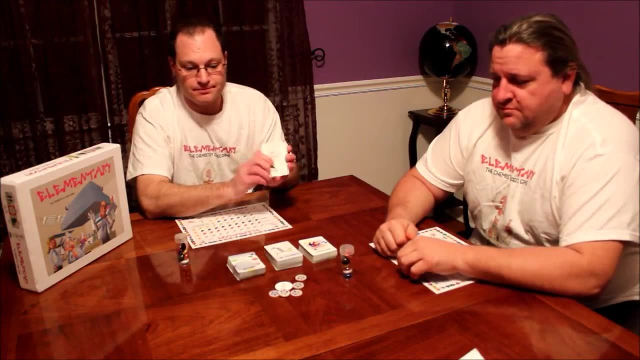 This is your element cards here. It's about 62 of these cards And these are for the compound marketplace which we'll set that up, And you'll also receive about four of these labs, So they're going to have where you're going to keep all your little elements. 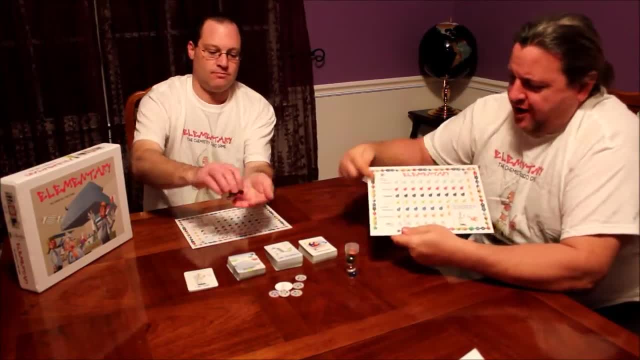 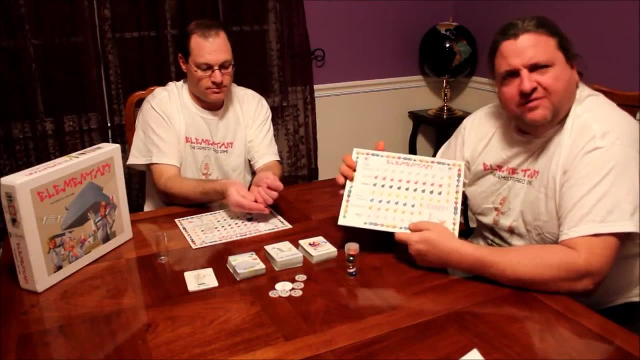 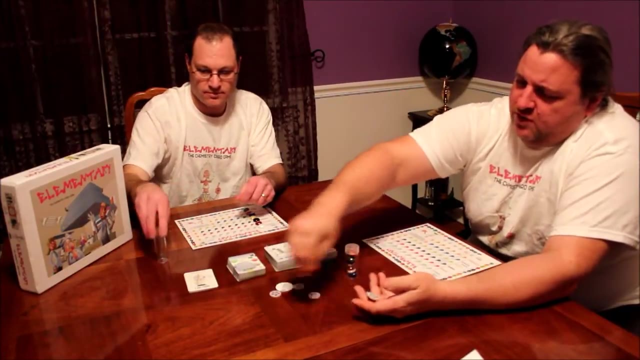 It's where these little tokens are going to have. You've got a scoring track going around the whole board. It'll give you the elements, the common ones. So, yeah, it gives all the explanations on your little laboratory And yeah, you come with these five little wooden player actions. 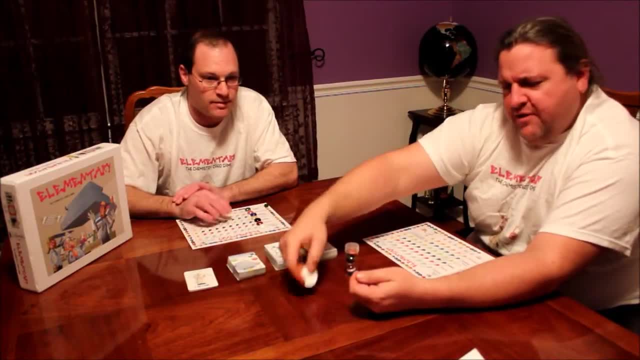 So everyone's got five actions. So you've got five of these And you've got a little player. It'll be your first player marker. So we're going to get this set up and then we'll give you a little rundown. 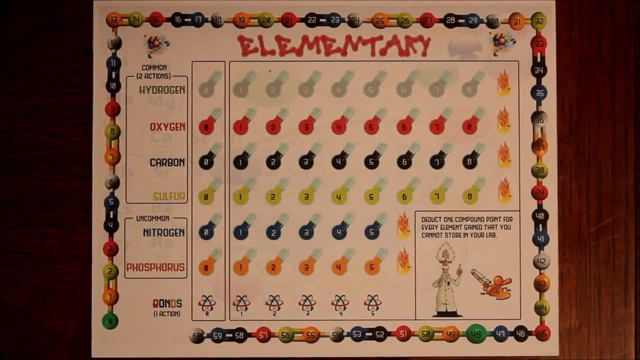 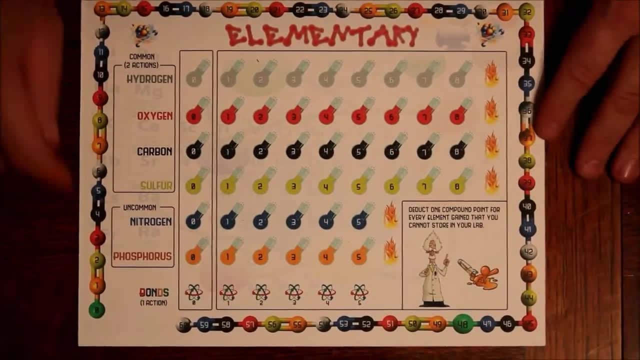 Okay, So the object of elementary, of course, is to get the most victory points out of all of your against your opponent. As you can see, here's your lab. Everyone's going to get one of these labs And around is going to be the score tracker. 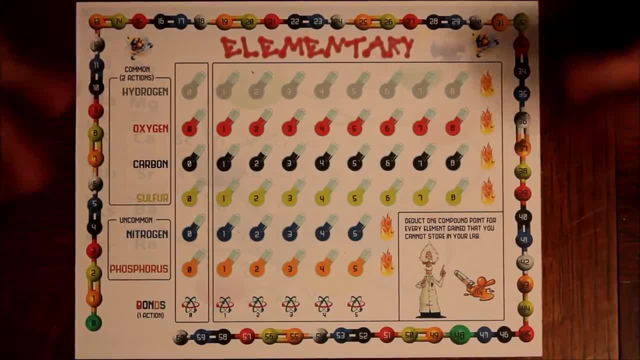 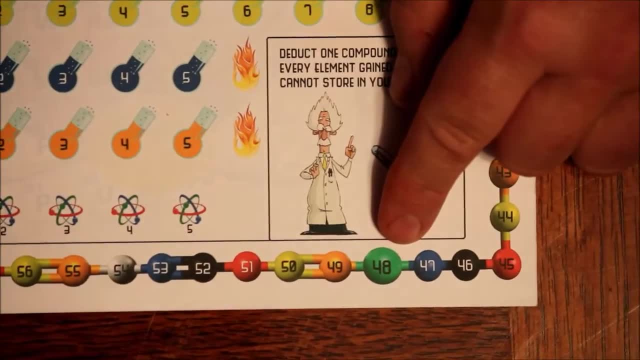 So what you're going to do is you're going to be trying to collect these compounds, which we call compounds. These are the compound points And the first person to reach 48, which we kind of determined the atomic weight of titanium. Don't ask why, I have no idea. 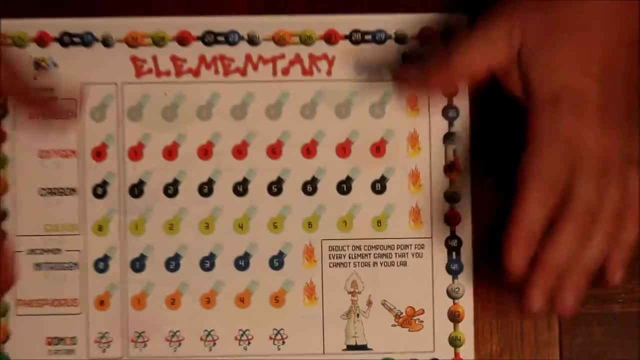 But 48 sounds like a good number. So what you're going to be doing is, when you set up your lab, they said you're going to get your little components here. So we have this little. everyone's going to have a different color. 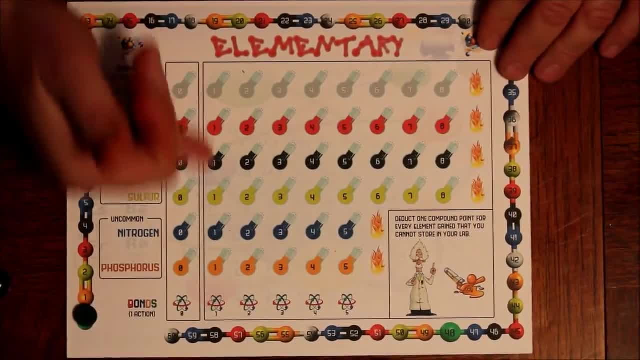 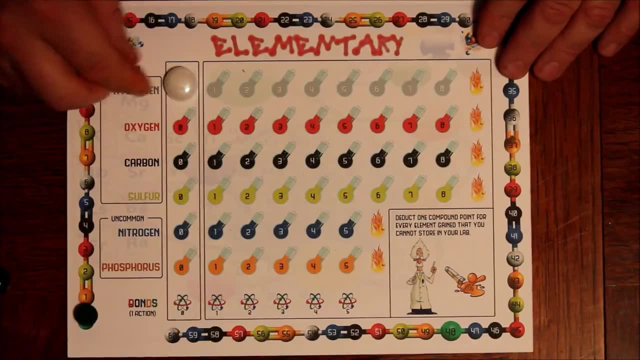 And you're going to put it on zero in the score track And they're going to have each of these. you have elements, So you're going to have hydrogen. you know they're each color coded, So the white one, which is, represent hydrogen. you know everyone's going to start it at zero. 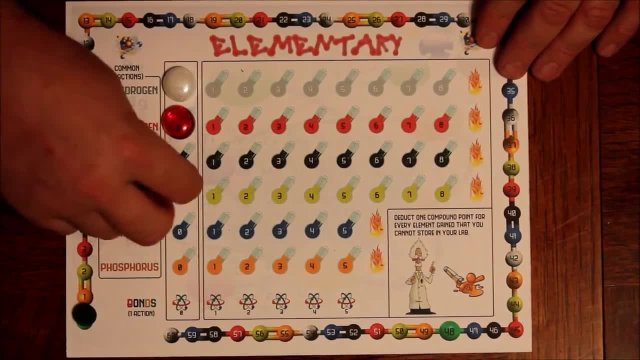 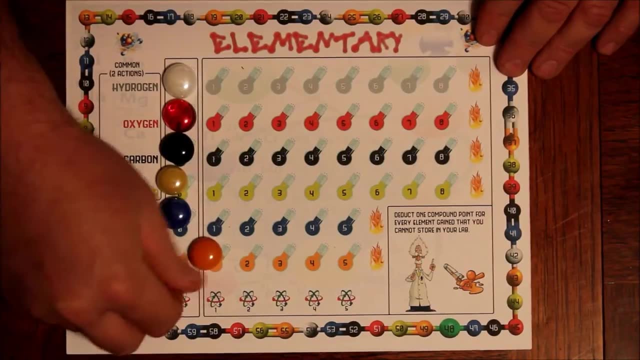 So you put, you start it at zero, with zero, With all the elements. so there's oxygen, there's carbon, there's sulfur, And then you have these other ones, you have nitrogen and phosphorus, And then the other one you have is bonds that we're going to be using to do compounds. 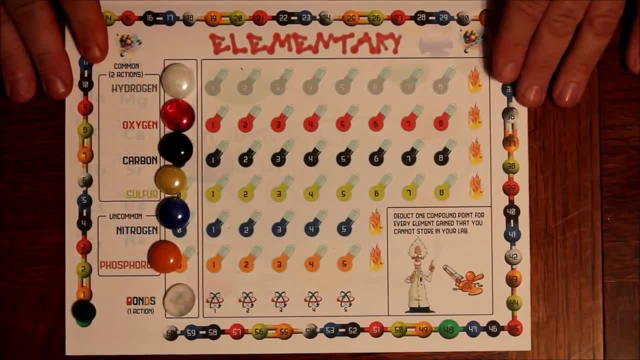 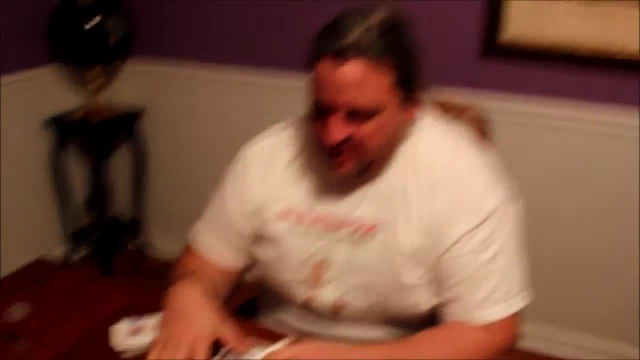 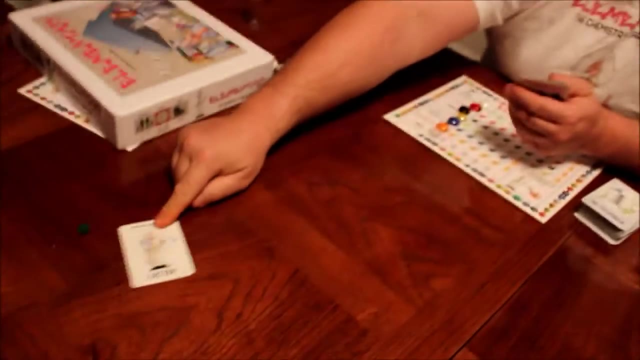 So then, all your, your lab's set up, you're getting all ready to roll, Okay, so now that everybody's laboratory is all set, ready to do some science stuff, we're going to put out the compound market. So we're going to take the compound market. 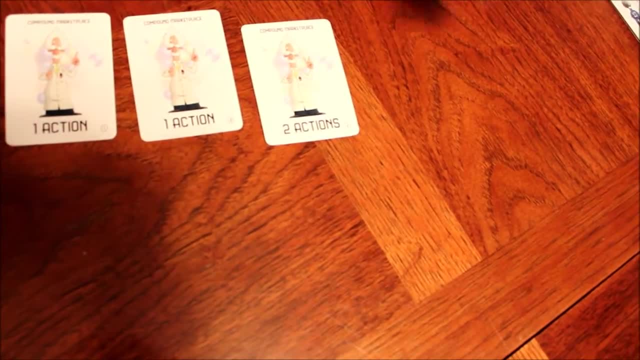 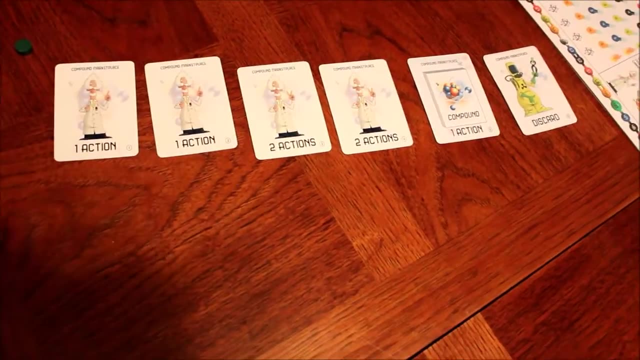 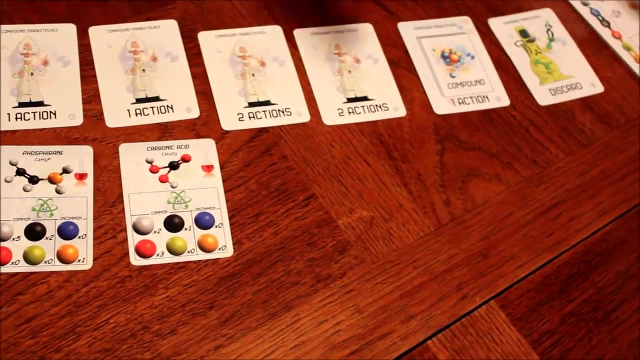 So there's going to be: these cards come out, these four cards come out and that one. So what this is going to do is you're going to put your compound cards, which is basically you're going to try to get these, to try to complete them and complete, get some points. 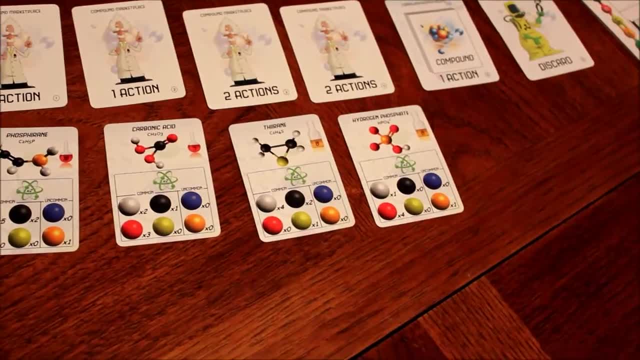 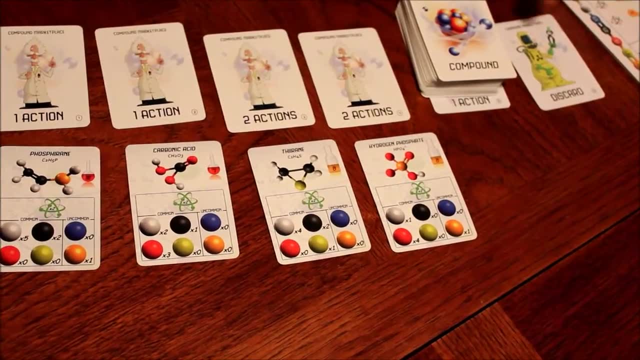 So these first four go here, then the entire deck, the compound deck, goes on top. So you got a draw deck, you got your, you got your compound marketplace with the four compounds and you have a discard deck. So, And then the last thing you need to get rid of, that goes right there. 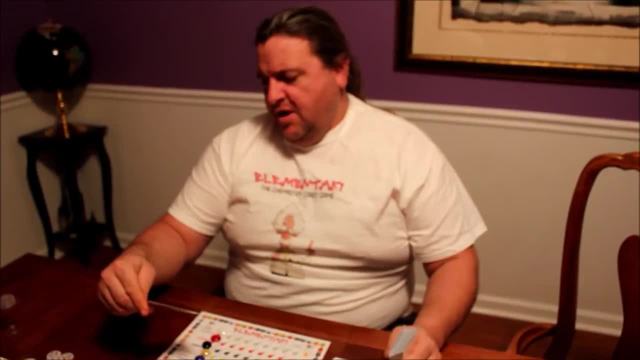 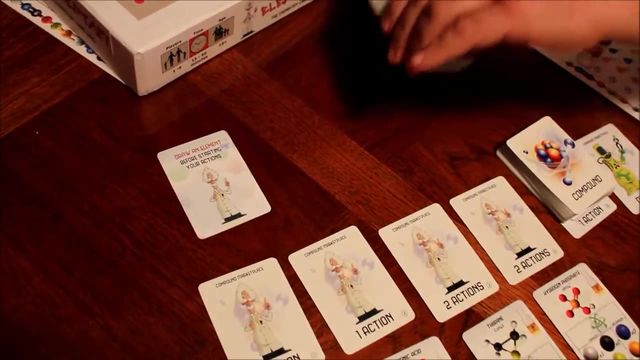 Okay, So after the compound market's there, the compound market's all set, you you're going to put out your elements And these elements you're going to use to kind of make these, make these compounds. So you know you need different types of elements to make different compounds. 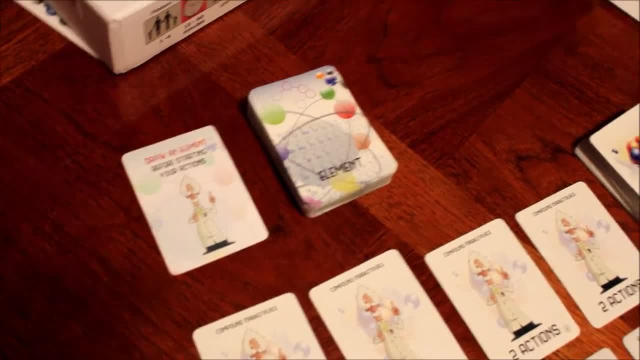 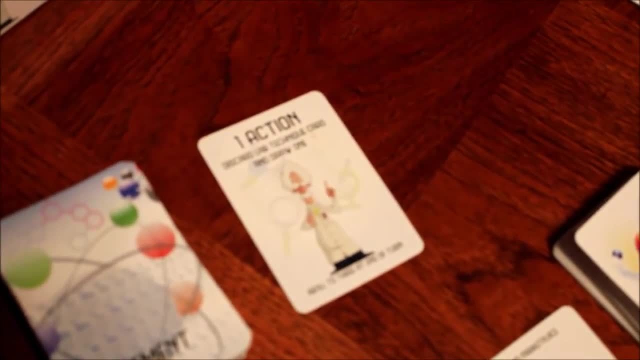 So you have your element draw deck, which is right here, And then the other thing you're going to put out is one more. you got one more lab technique. So these are the lab techniques. So you use to kind of cheat the game kind of a little bit, kind of break the rules a. 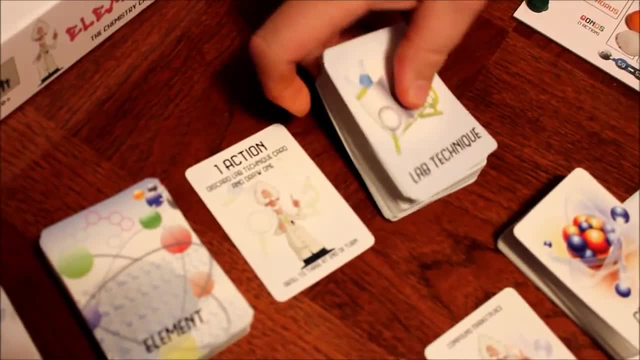 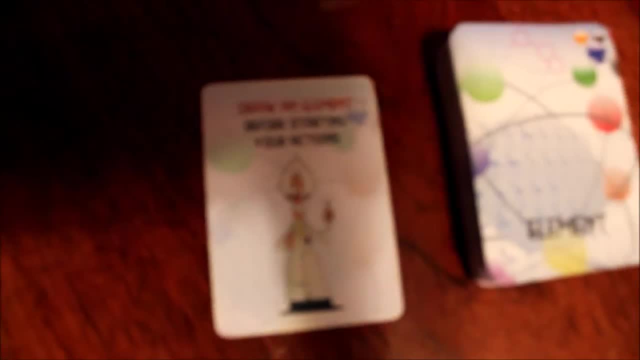 little bit. So you're going to be putting that down next, there, There, And make sure everybody you know nice little room so you can have a little discard pile. And then you're set. You got your compound marketplace, You got your elements to to pick up and your lab techniques. 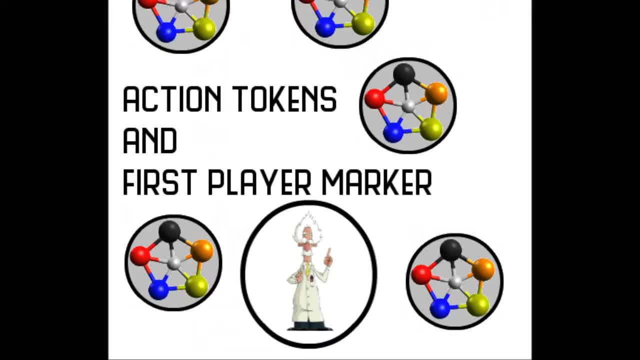 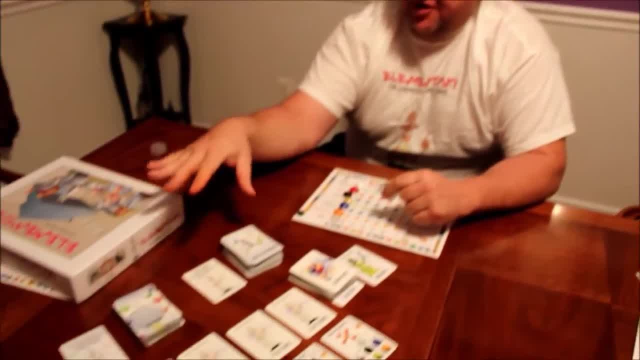 And you're all set to play and do some science. So, after everything's put down- your lab's out, you got your compound market, you got all your cards out- The most important thing to do is decide who that first player's going to be. 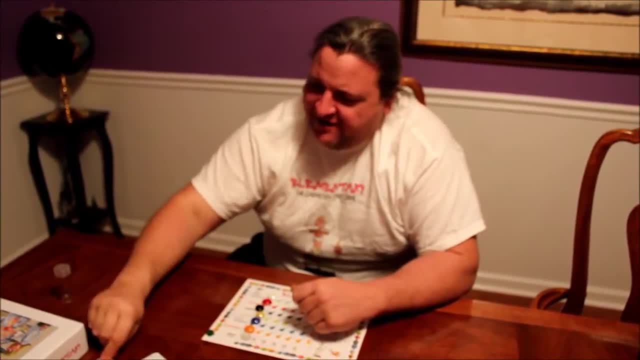 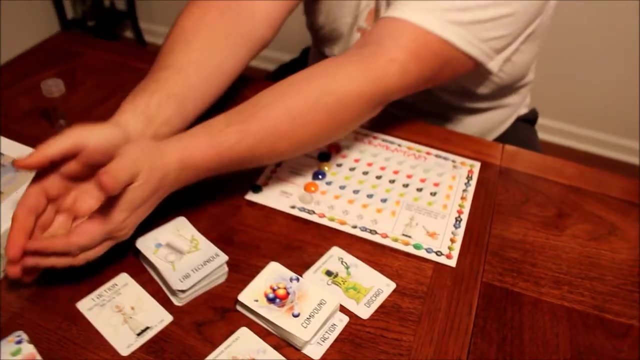 Do it any way you want: Oldest, youngest, Just decide, And then get it the first player mark And then give them all the five wooden discs, If you're all action, action discs, And then now you're all set to play. 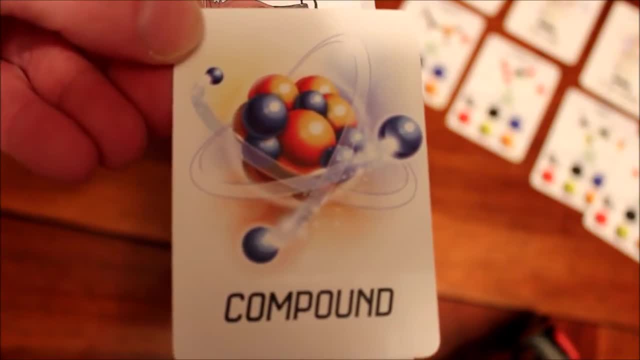 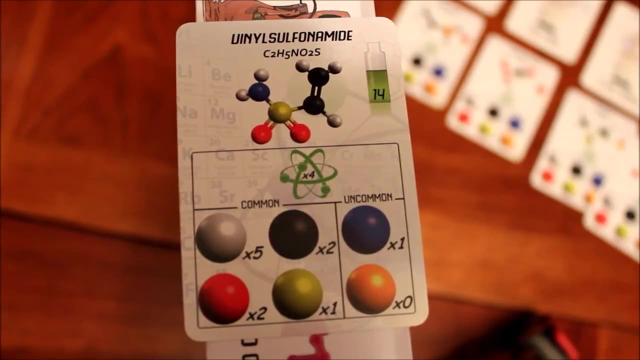 For the compound cards. I'm going to give you a breakdown of how to actually read one. So we have a card here: vinyl sulfamide C2H5NO2S. We have the formula here, The ball and stick model, just for fun. 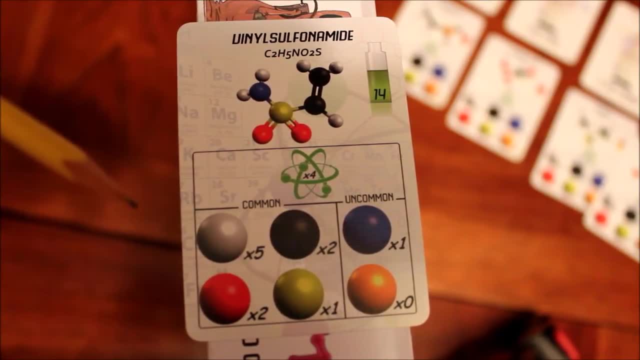 The formula is down on the bottom over here And that's what you're trying to collect on your laboratory. So the bottom left corner. we have oxygen, two of them, Hydrogen five, Sulfur one, Carbon two. 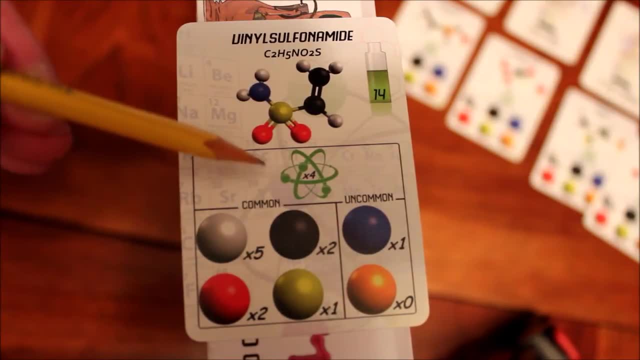 Phosphorus zero And nitrogen one In the middle. this symbol is for the bonds you need to collect to complete the compound. Four of those In the upper right hand corner. that's the number of compound points you'll receive when. 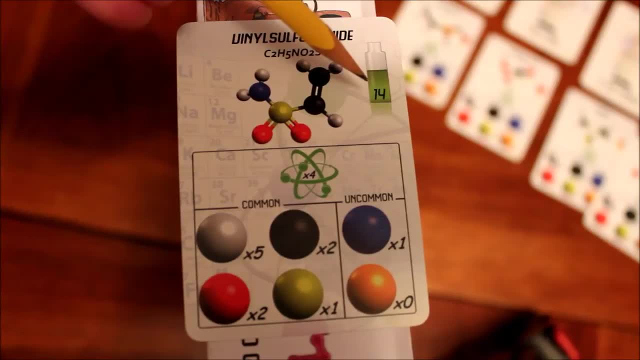 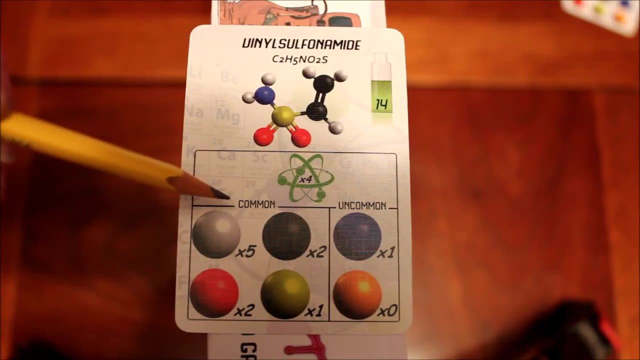 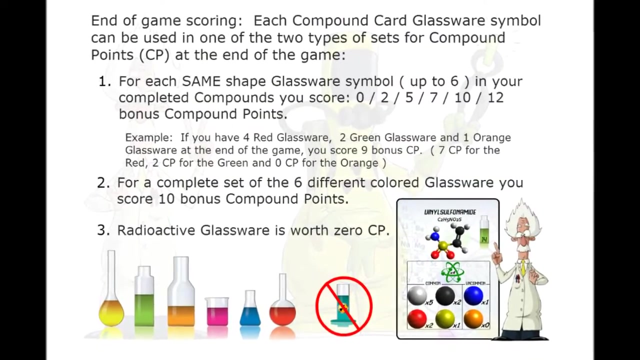 you complete this compound. So this particular one is 14 points On the left hand corner down here. these four elements are the common elements. On the right hand side, your nitrogen and phosphorus. those are your uncommon elements. They're harder to get in the game. 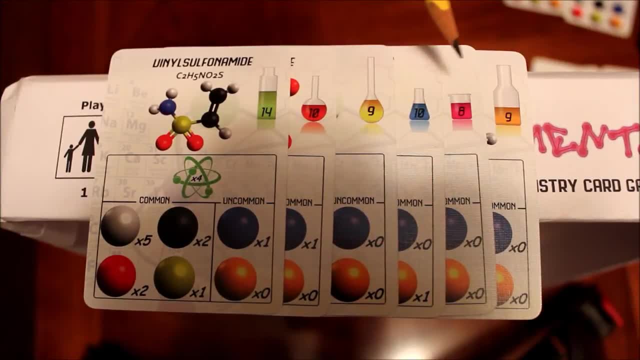 If you look in the upper right hand corner of the compound cards, you'll see these different glassware symbols For the end of game scoring. what you're trying to do is one of two things. You can try and collect a complete set of six, which will give you an extra ten bonus. 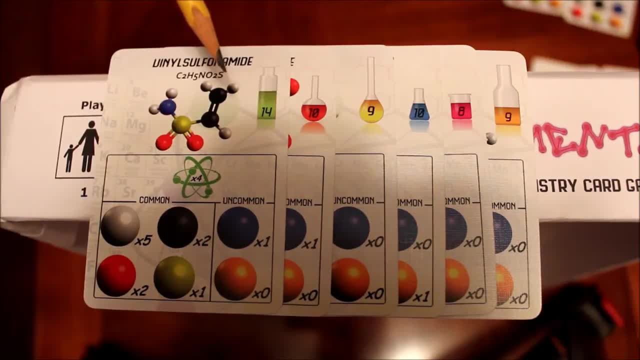 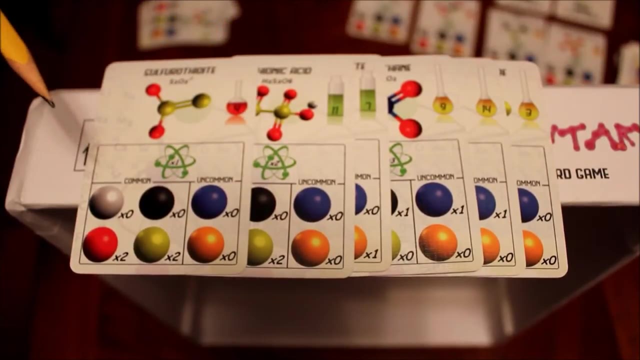 points Or you can try to collect the same image over and over again to get a multiplier of points. For each same shape, glassware symbol, up to six in your compound. you're going to have your completed compounds. you score zero, two, five, seven, ten, twelve bonus points. 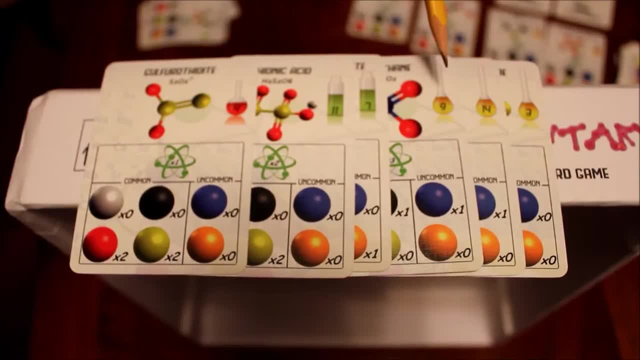 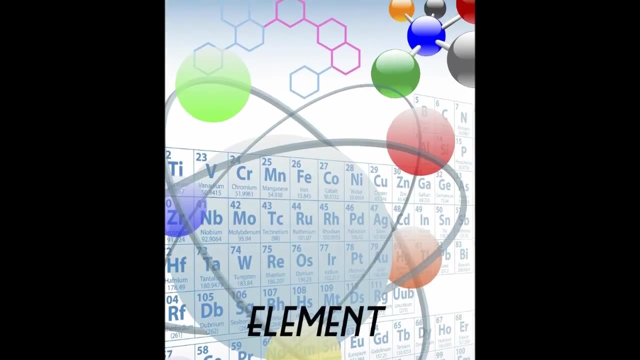 So, for example, here you have three yellow glassware that's worth five points, Two greens that's worth two And one red that's worth zero. So you get a total of seven bonus points at the end of the game. 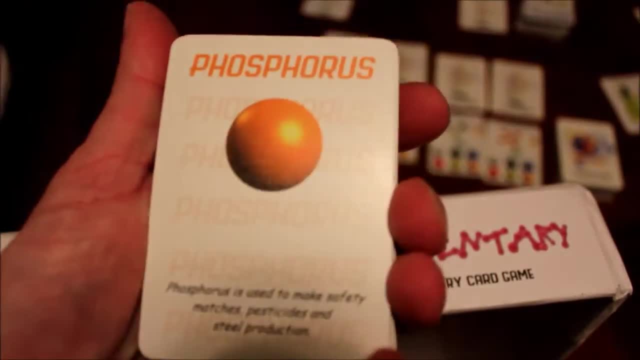 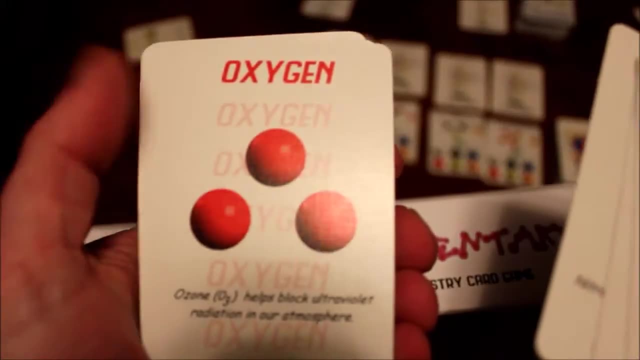 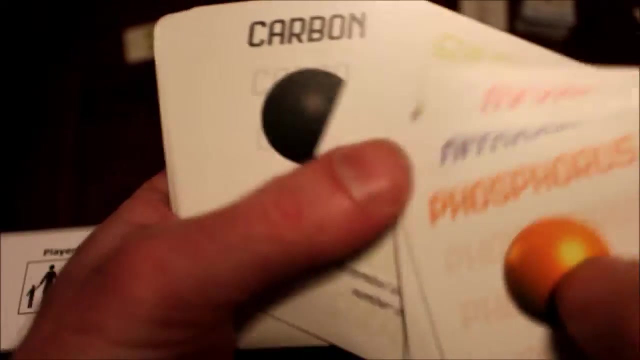 Here's a look at the element cards in the game. So you've got phosphorus, hydrogens, nitrogens, you've got your triple oxygen, an oxygen which will allow you to take another element card, sulfur, carbon and so forth here. 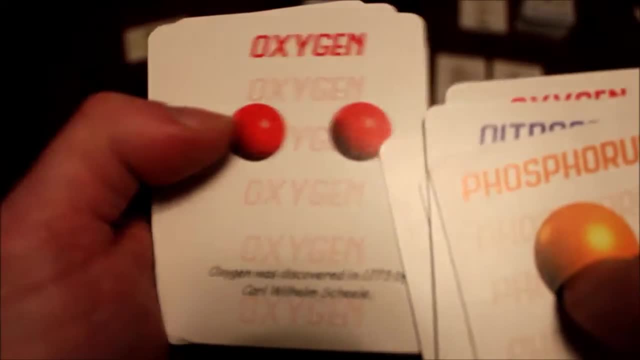 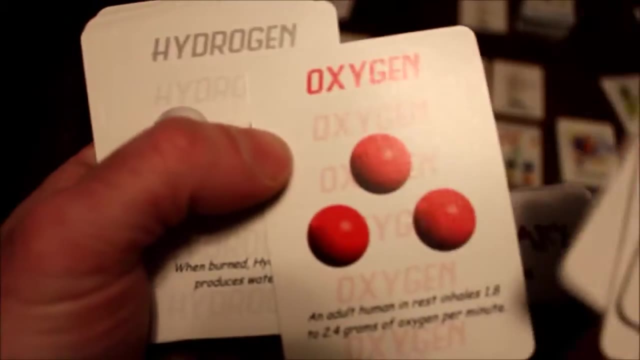 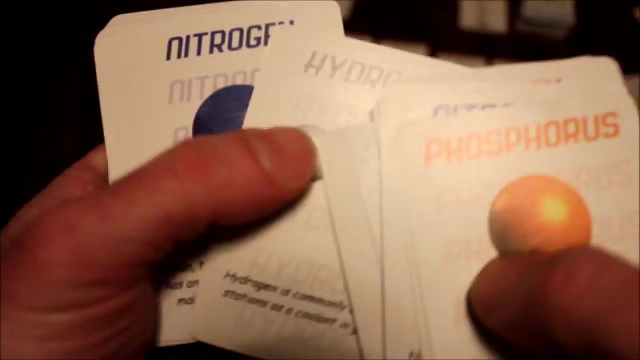 The hydrogen and oxygen have ones, twos and threes. Here's a lab fire. All players lose one active player's choice. The phosphorus and nitrogen are very hard to get. There's only six of each of those in the deck. single elements: 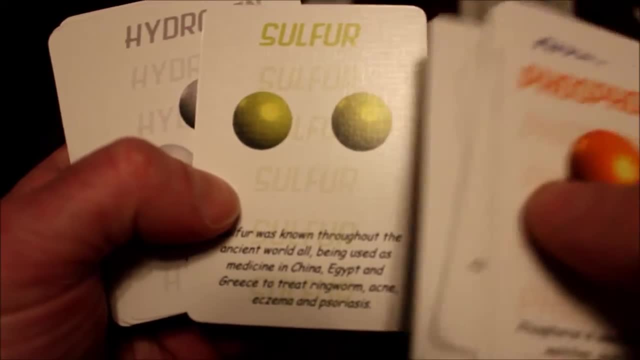 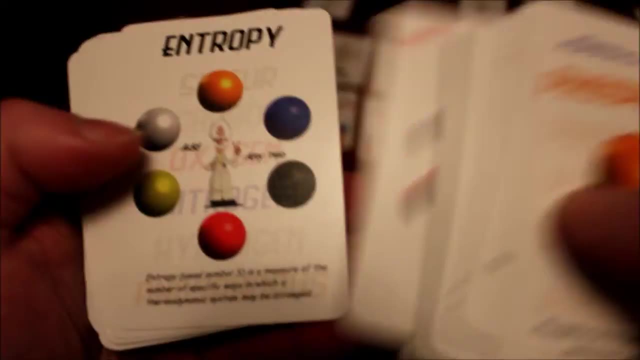 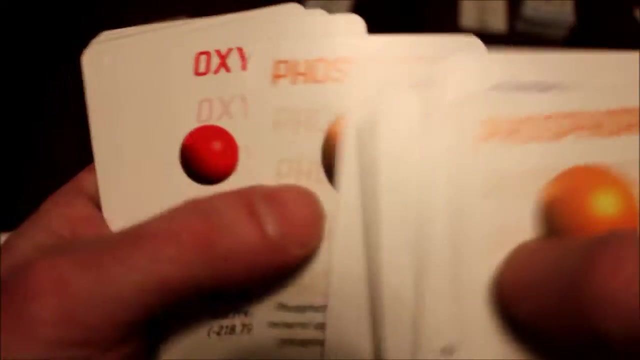 And the sulfurs. there's eight cards of sulfur and eight cards of carbon, with ones and two elements on those. There's also wild cards such as entropy. This will allow you to take any two elements And let's see what else we have here. 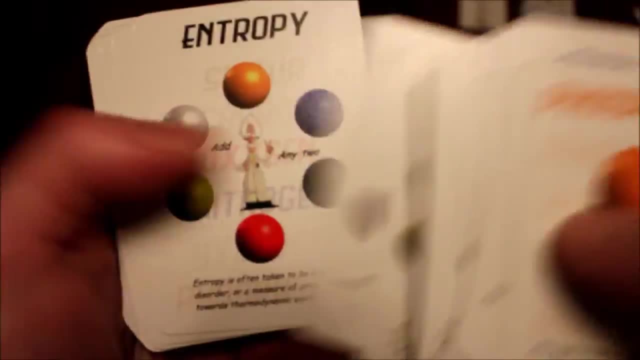 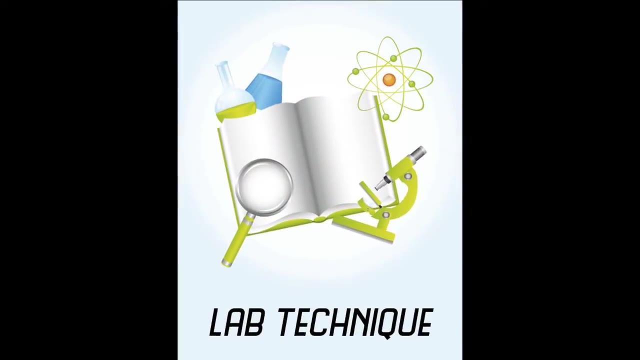 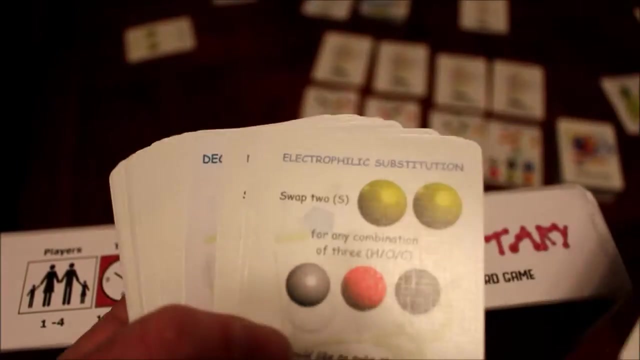 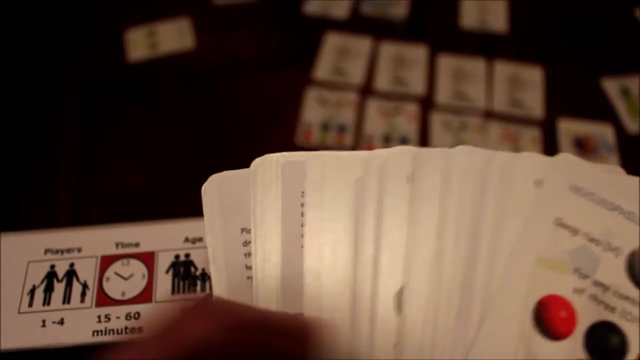 And enthalpy any one element And that is the element deck, The lab technique deck. This is approximately 80 cards. This is going to allow you to get elements quicker on your board. It's going to help you to get actions in the compound marketplace quicker from the discard pile. 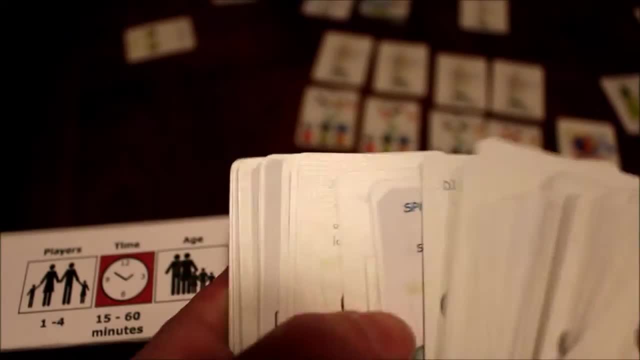 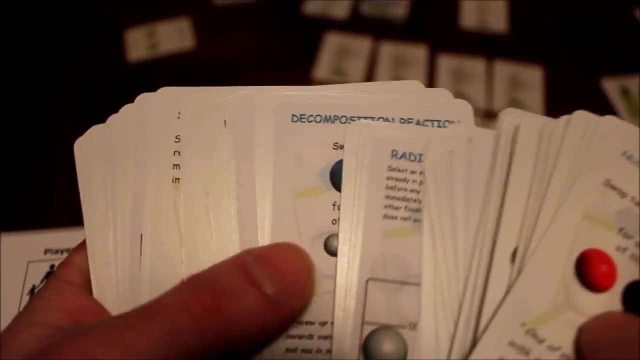 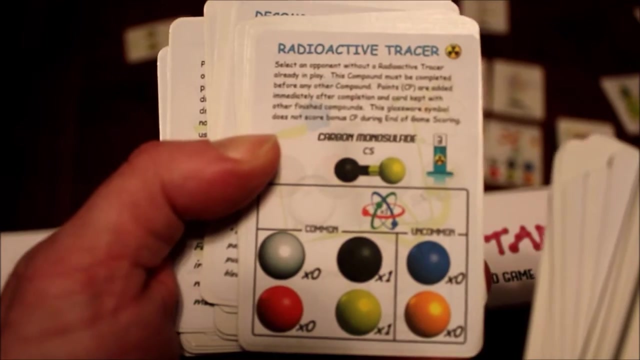 All kinds of ways to play cards in the compound. You can play cards against other opponents like a take that Finishing compounds. You'll be able to play certain cards that will help you finish compounds. There's also the ability to play compounds on other people and force them to do them before they can complete other ones. 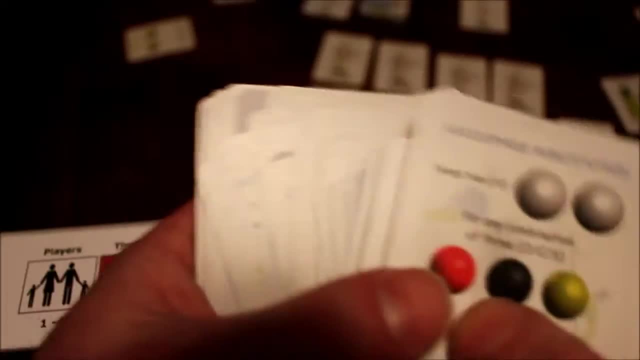 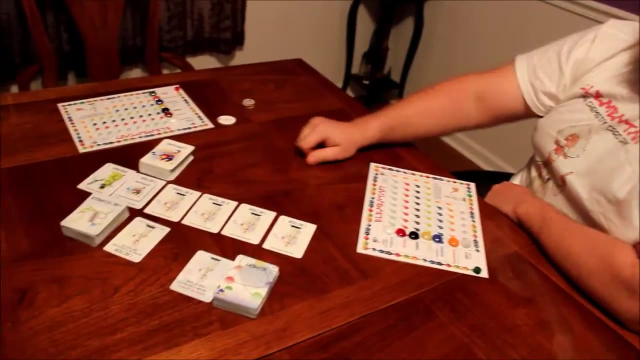 And we'll go through these cards, as we're actually playing the game in more detail. Okay, so now you've got the basics down, You've got your components out. We'll set this up in a minute. Consult the rules. Apparently, Young's player is going to be the first player. 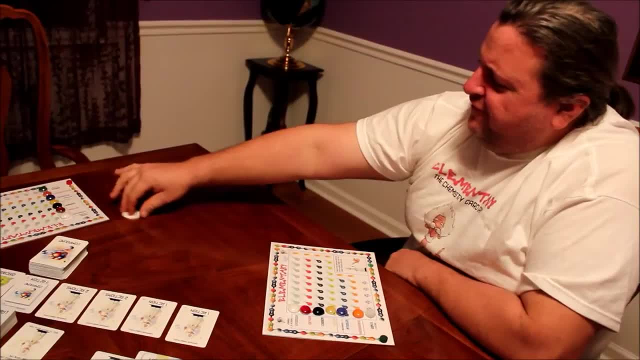 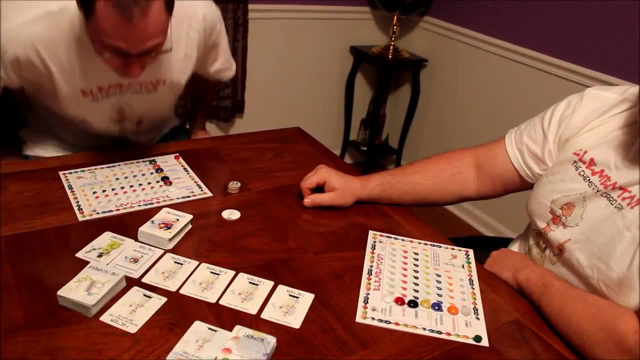 So he's going to be the first player, So he's going to get the first player marker And he's going to get his five actions. We'll set this up and we're going to give it a go. All set. Yeah, all set. 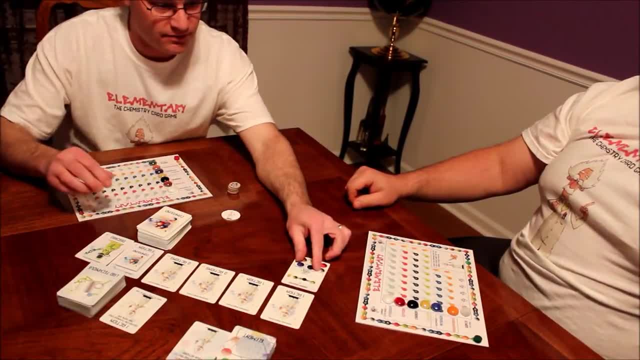 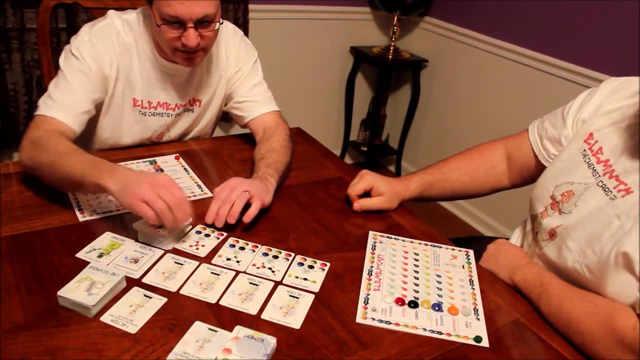 All right, So let's set up the compound marketplace here first. Okay, I'm going to get my old man glasses on Carbon disulfide, phosphorine, thyrine, hydrogen phosphate. I'll take three, So the first player gets three lab techniques. 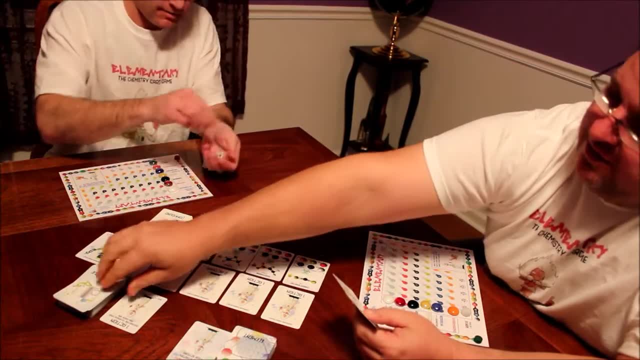 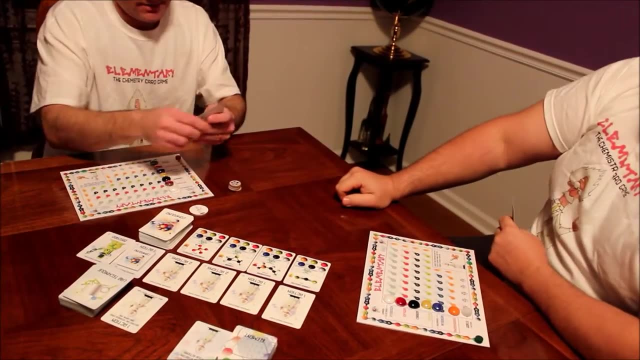 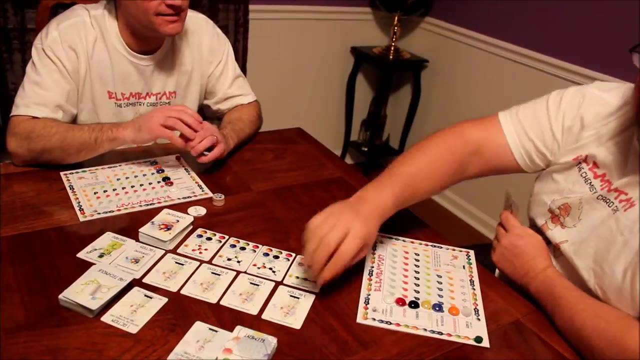 And I'll draw my three lab techniques Now, finally, we're finally ready to play. Okay, so we've got five actions. Here's your hand. Here's the start player. All right, Okay, So what you always do on your first turn is you will always draw an element card. 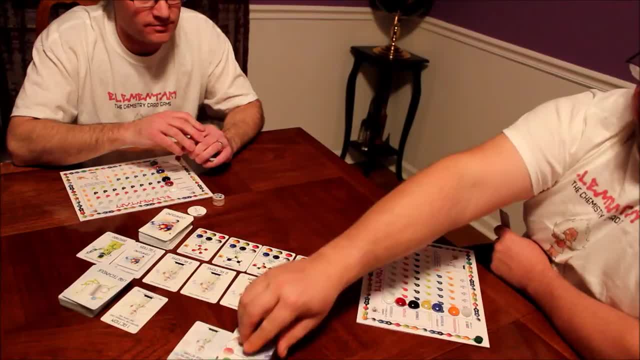 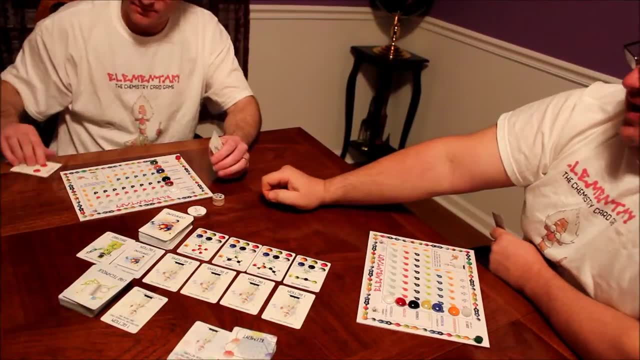 These are basically to get. when you draw an element, you're basically going to flip it over. So for him I'll just do it. for him I'll flip it over And you can see it shows two oxygens. So what he does on his lab, he gets two options and discards it. 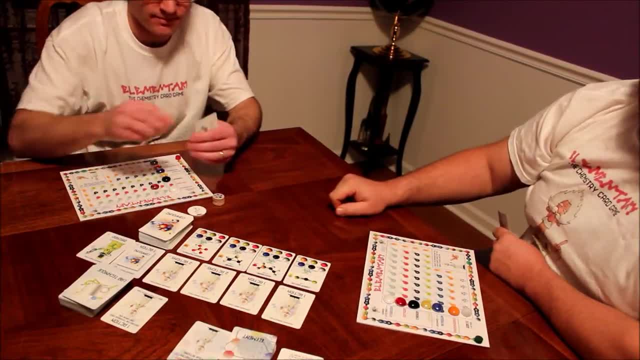 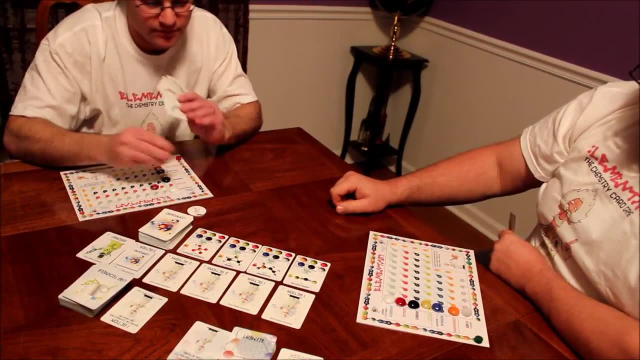 So he's able to put two up there. So that's how you get your elements. So now you can do your actions, or a lot of actions you can do. Okay. So for my first action, I'm going to purchase this one action card from the compound marketplace. 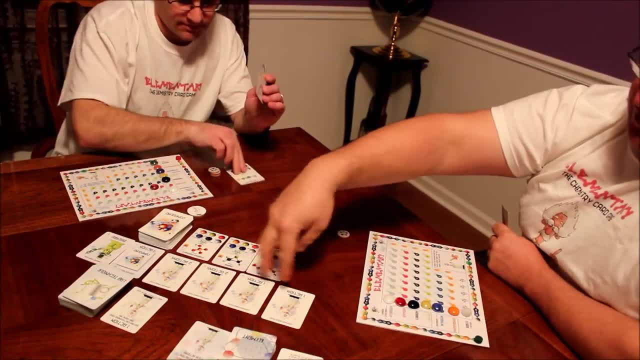 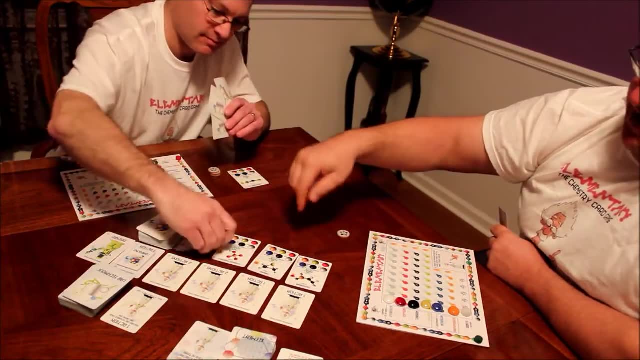 Yep. So what happens is carbon disulfide. So what happens is: so each of these are going to have. they're going to be one action, one action, two action. So what these are going to do, if you buy an action, notice how they all have different number of actions. 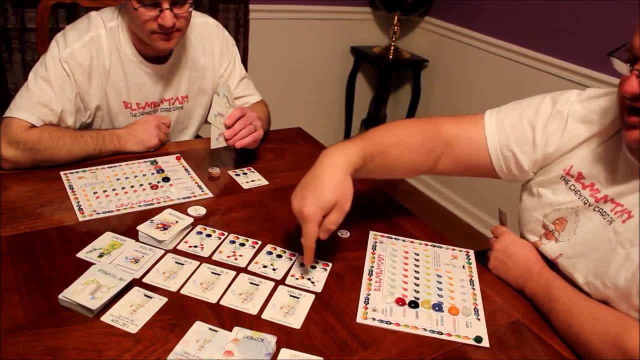 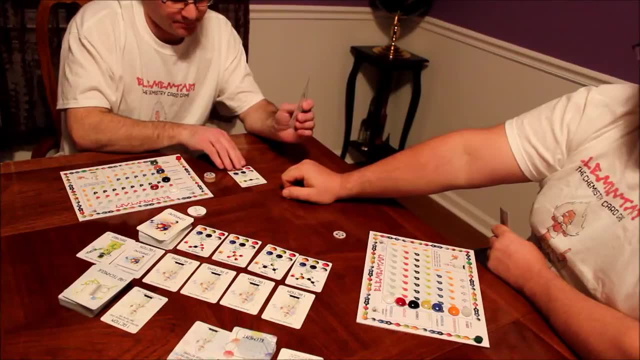 So if you wanted this action, you would have to pay two instead of one, But since he got the one that cost one action, it only cost him one action. Okay, So from here That goes into his pile and the other thing there that goes into your to your. so this is what the compound he's working on. 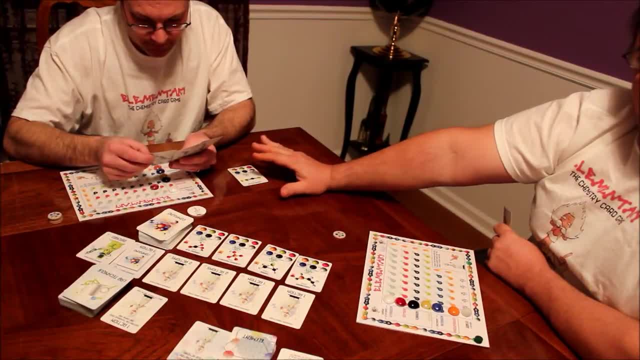 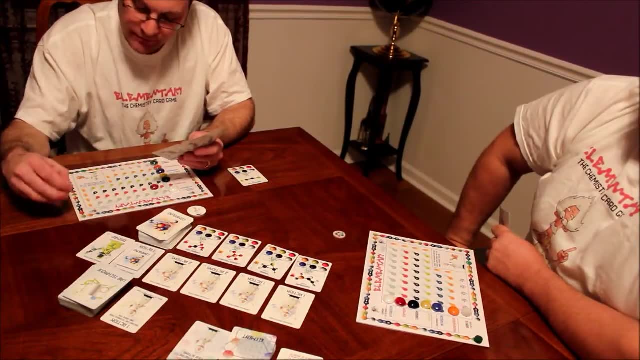 And you can only. you're only allowed three compounds in your little set area here. If you ever go over three, you have to choose one and then discard it. Okay, So I have four actions to go. You have four actions left. 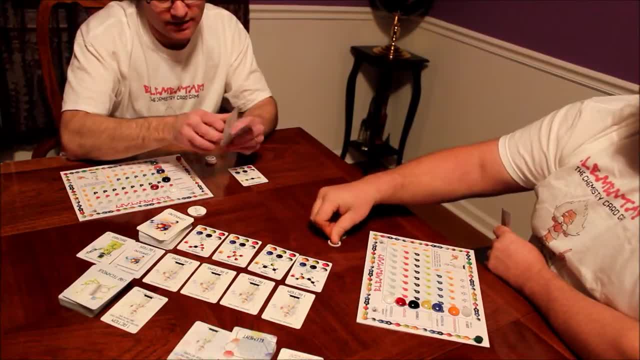 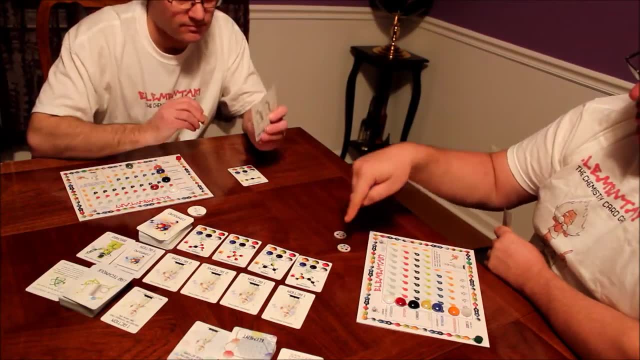 Right, And so I'm going to play an action. Quantum chemistry: add three bonds to my lab, Right. So anytime you play a lab technique card, One, two, three, So yep. So anytime you play a lab technique card, you always have to spend an action. 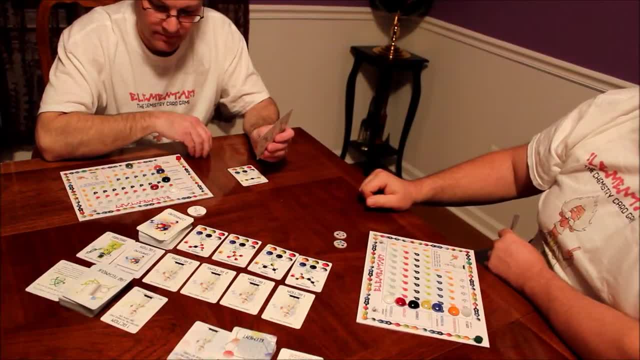 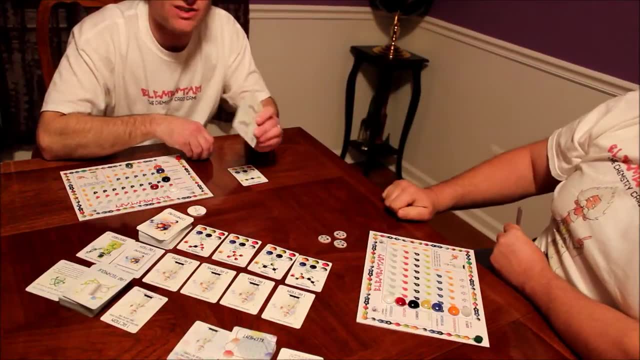 Do with the caption, So his he's able to get three bonds for spending an action. That's pretty good. Okay, I'm going to spend another action, Idea being: you want to use these cards up as often as you can, because then you can refill them to your hand of three at the end of the turn. 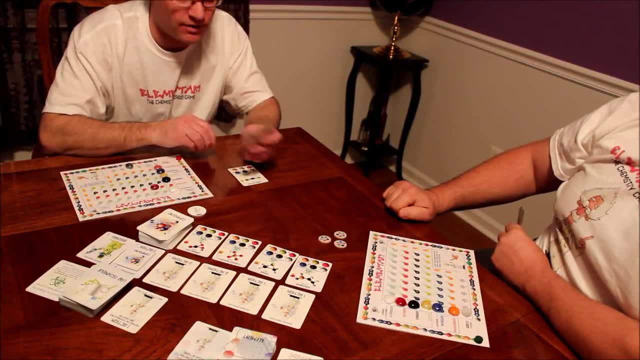 If you're holding onto the same cards, you're refilling them. Okay, It's really it's hard to to move forward. So for that action, I am going to play spontaneous vision and swap this card for any one common element. 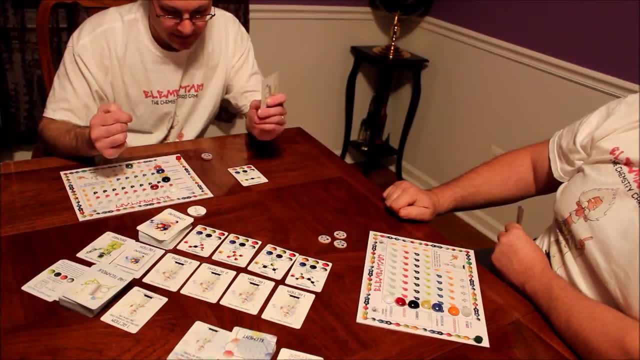 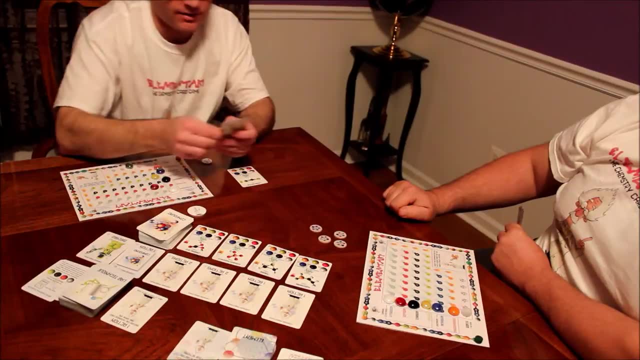 And I'm going to take a. I'm going to take a sulfur because I need a sulfur to complete this compound. For my fourth action, I'm going to play oxidation. This allows me to swap two oxygens for any three: hydrogen carbon or sulfur. 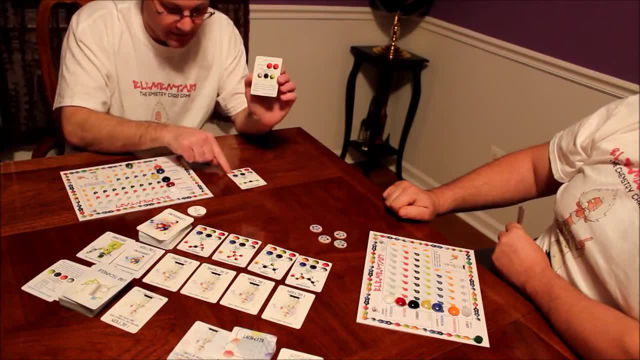 So I'm going to remove my two oxygen and I'm going to take a carbon, A sulfur And a hydrogen, One of each action I'm going to take. I could have taken two and one, but in this case I wanted to take one of each. 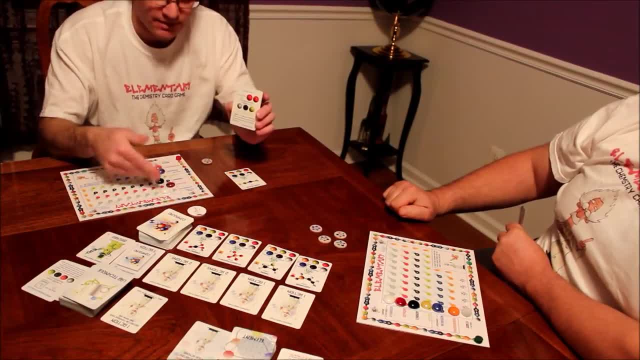 I'm going to discard that And for my last action, I'm going to go and immediately complete this compound. I have everything I need here, So let's see I need, starting from the top. here it looks like I need a carbon. 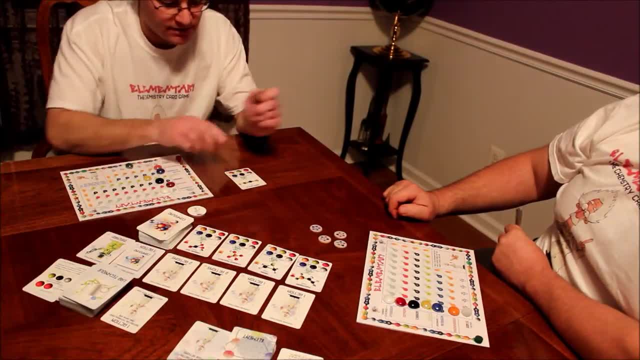 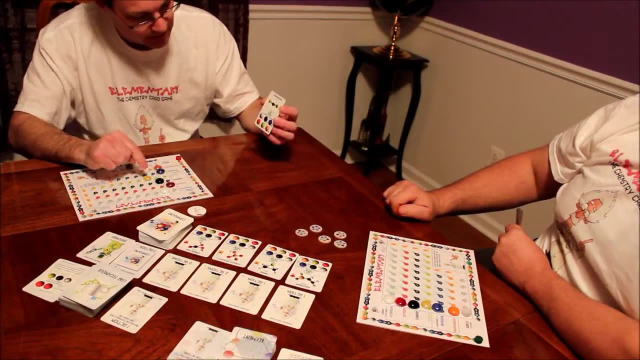 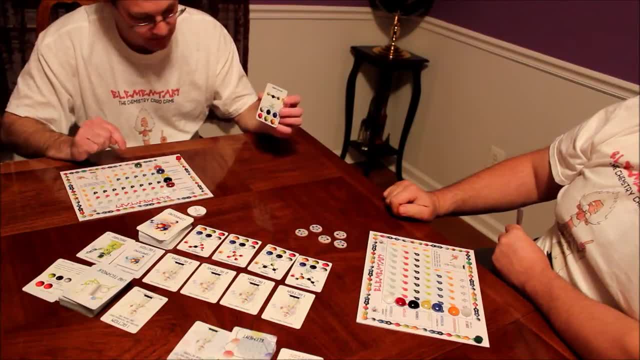 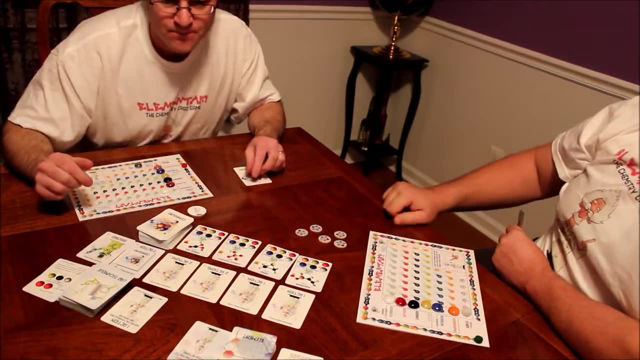 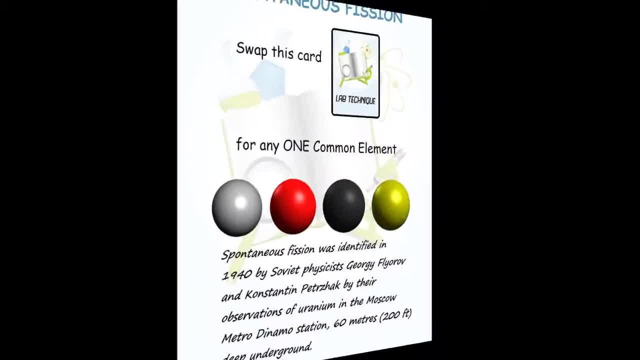 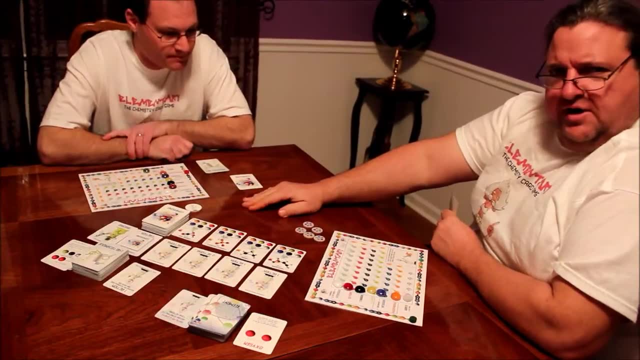 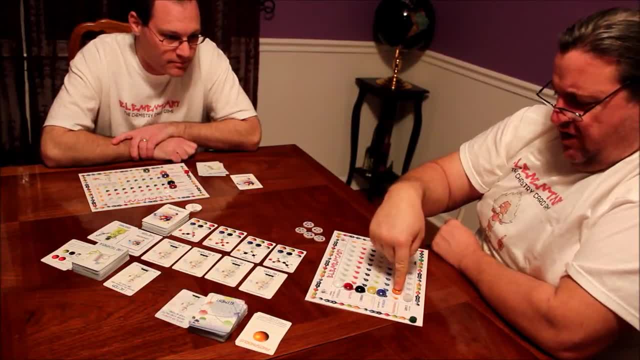 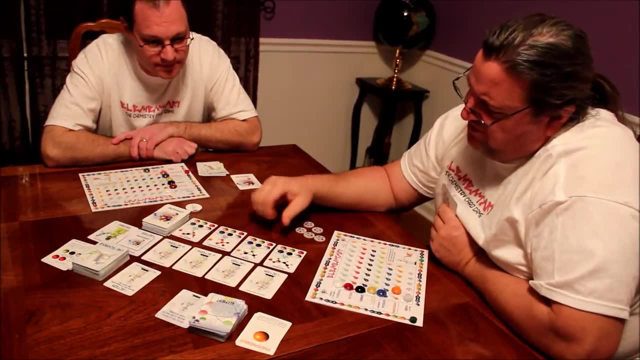 This one. I was able to get phosphorus, So that's usually pretty good, because these are the pretty uncommon ones, And okay. So what I'm going to decide to do is I'm going to look at the marketplace and say, yeah, I don't like any of the cards I see there. This one I have to. you know these. 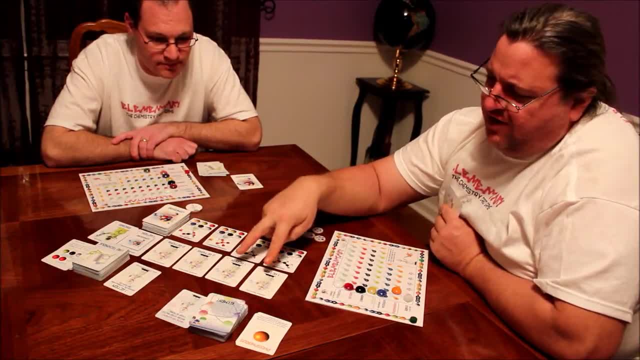 things are going to cost different actions. So if I wanted these two here, it'll tell you right here it'll cost me one action. If I wanted these two here, it would cost me two actions. I don't like any of them. So what I'm going to do is I'm going to use 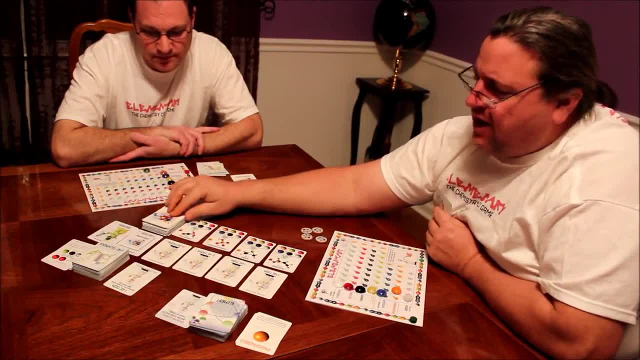 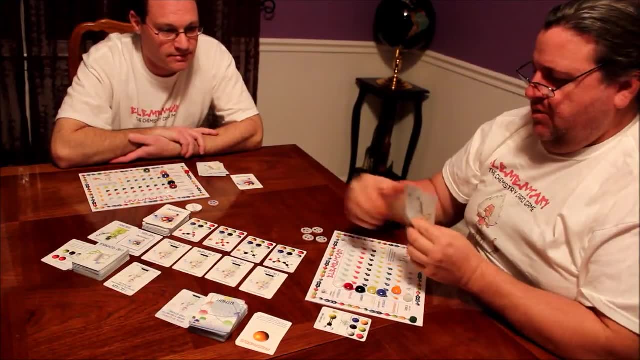 the one action I'm going to pay. one action. I'm going to take the top compound card right off the top And I'll put it right into my pile here. Okay, that looks pretty good. So for my second action, what I'm going to do is I'm going to play one of these lab technique. 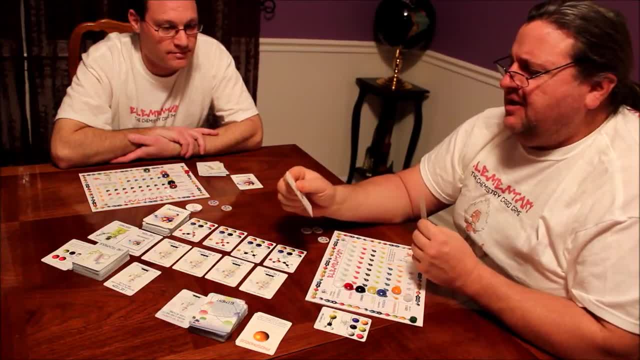 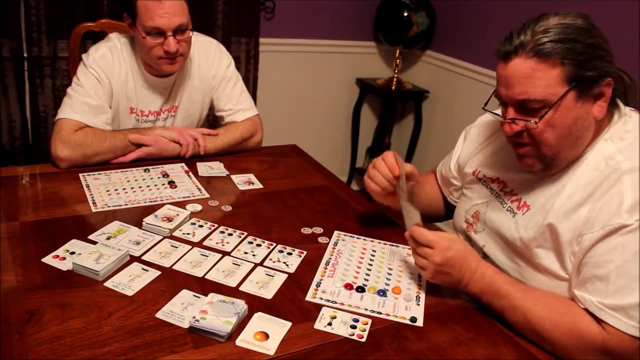 cards. This one's going to allow. it's called double replacement. It's going to allow me to add any two elements, any one I can choose, and then my opponent's going to get one. So I'm going to look at my card, where I'm kind of neat, So I'm going to add: I'm going to 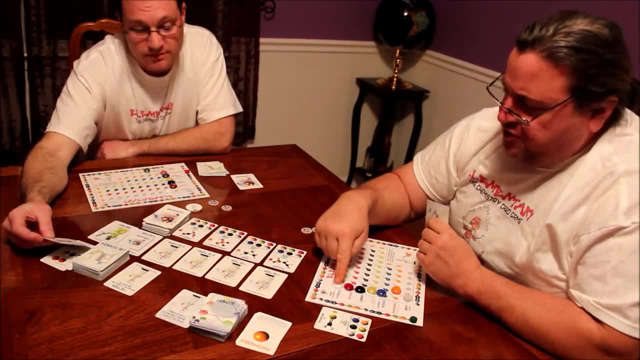 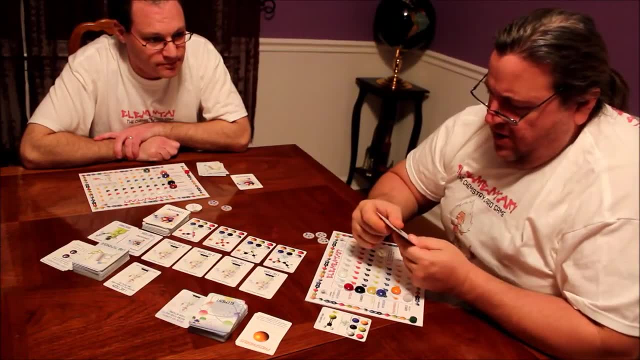 play it and discard it. So I'm going to add two hydrogen, and then my opponent, since the card says I'm going to add one And that's one. So I have three more actions. Well, look what I'm going to do. So what I'm going to do is I'm going to spend this. 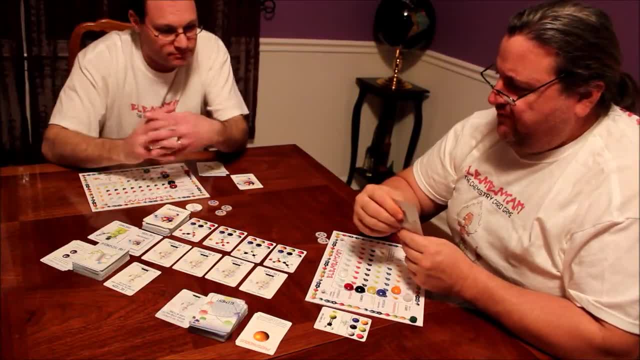 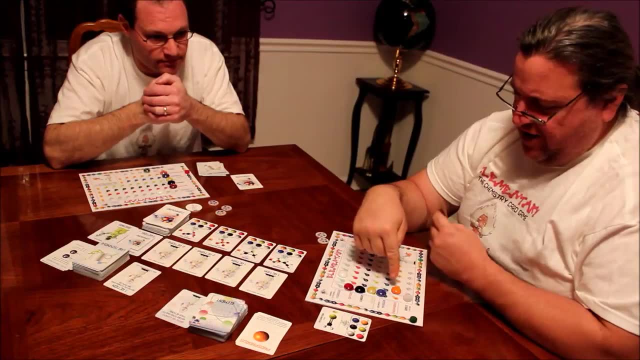 I'm going to play another. I'm going to play another lab technique card, So I spend the action I'm going to play. it's called the redox reaction. This allows me to do that. I can swap out the phosphorus that I just got, So swapping it. swapping means you're. 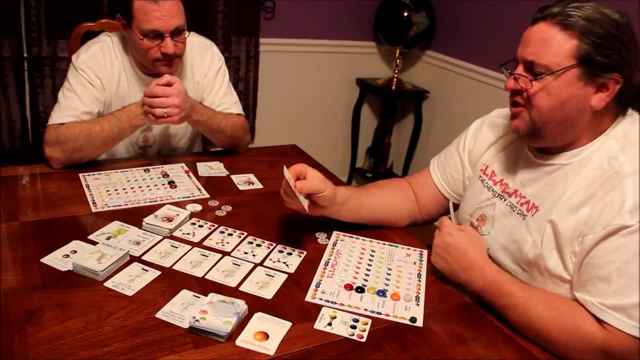 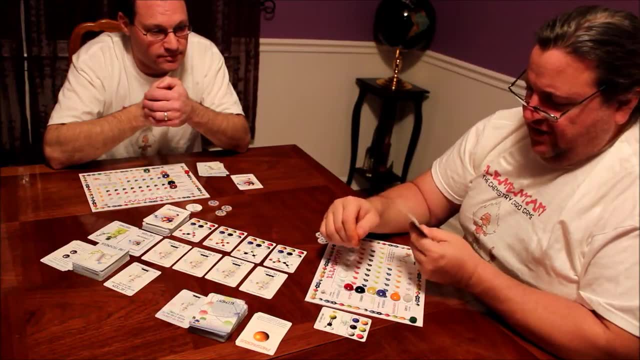 losing it. So I will lose that And this card is going to allow me to take any combination of any of the any three of the common elements. So I can take, you know, like three hydrogen, three oxygen or two hydrogen. 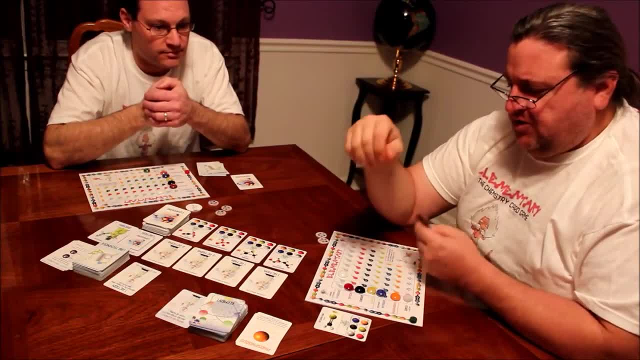 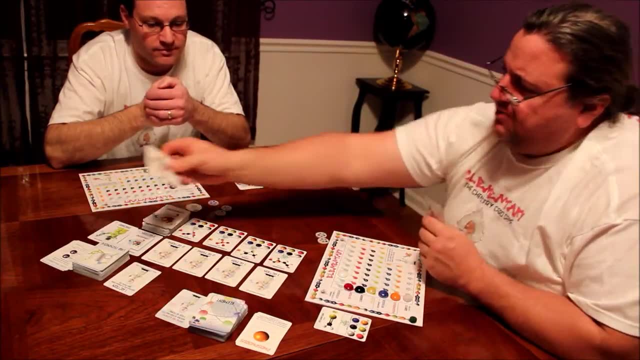 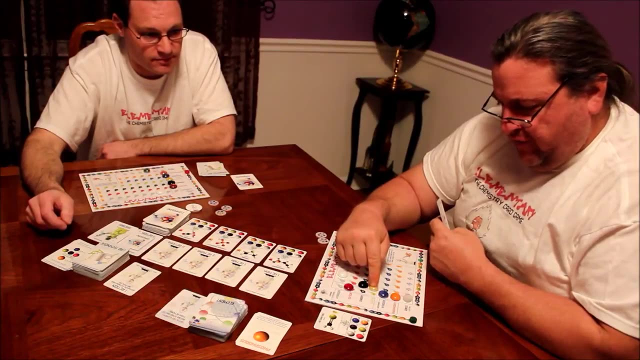 One oxygen, you know any, any of the common ones in multiple three. or it allows me to take the nitrogen So I can take the other uncommon element. So I'm just going to play and discard that, And then I am going to take one carbon, I'm going to take one sulfur and 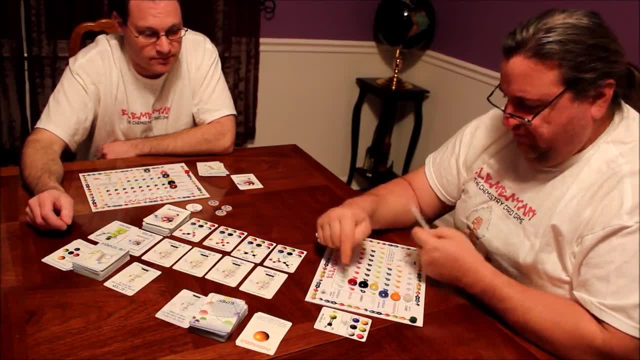 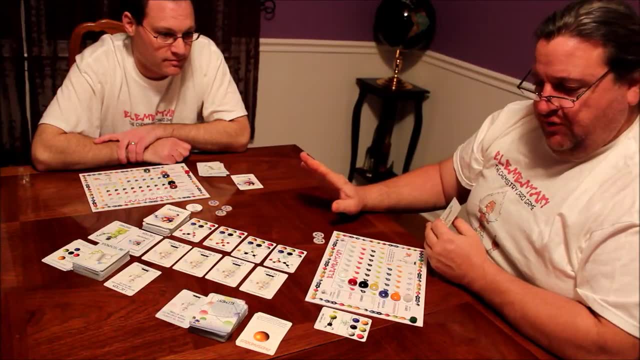 just for good measure, I think I'll just take, I'll take an oxygen. Okay, So I have two more, two more actions, And what I'm going to decide to do is what you do, what also you do for two actions. 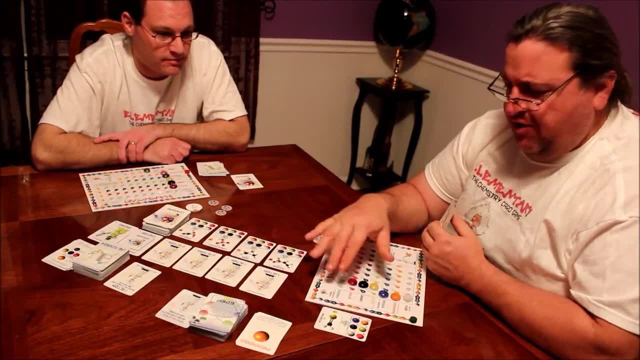 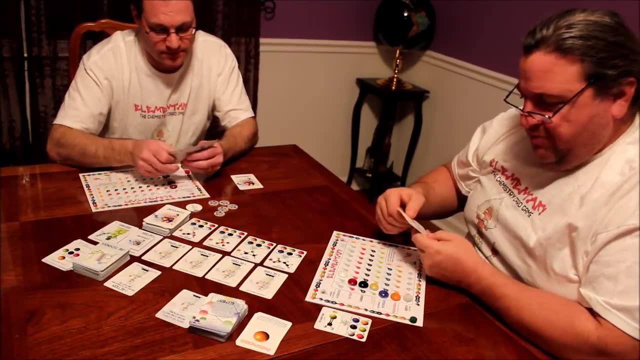 Is that you can buy any one of the common elements of the. so I can either buy hydrogen, oxygen, carbon or sulfur for two actions. So I'm going to do that, So I'm going to pay my two actions and I am going to go up in I don't know, let's see oxygen, So then I'll. 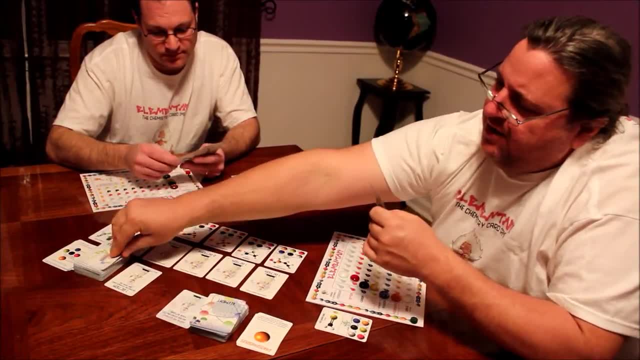 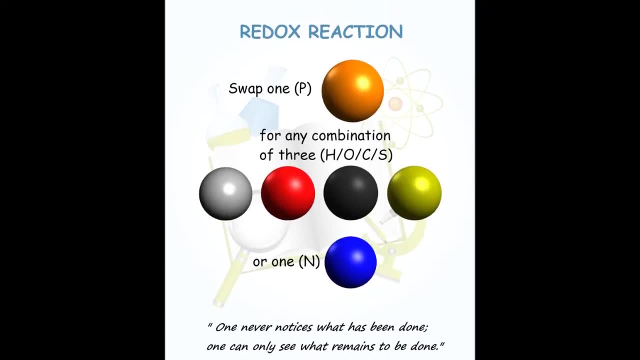 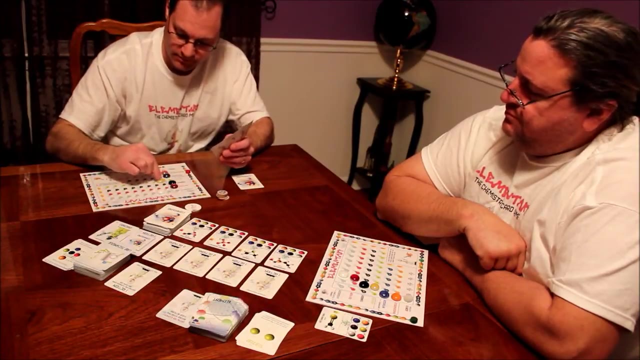 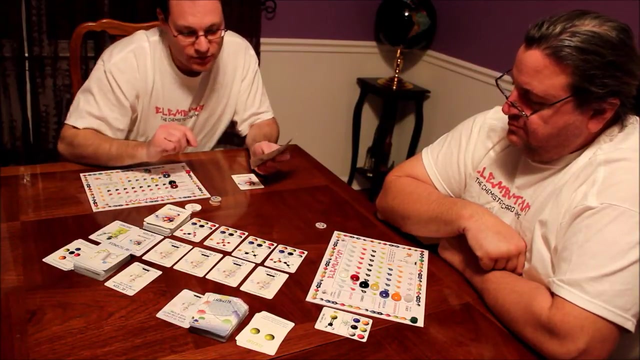 see, I only have one lab technique card in my hand. I'll draw up to three and my turn is over. All right, I'm going to draw my element: Mm-hmm Two. sulfur, Mm-hmm One- two. Okay, For my first action. I have no compounds here, So I am going to play the. 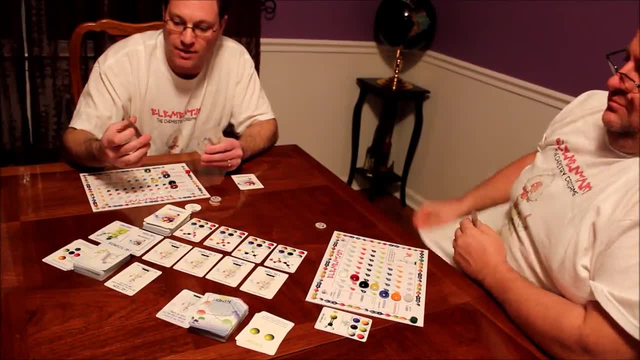 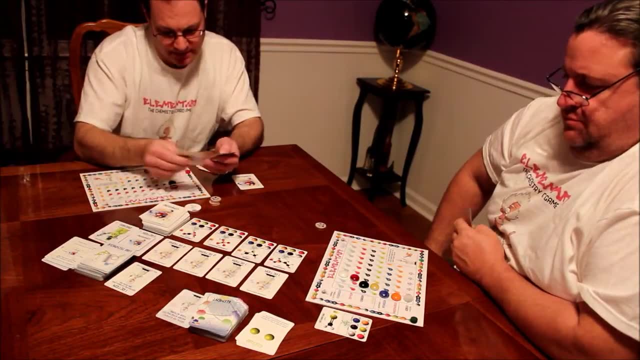 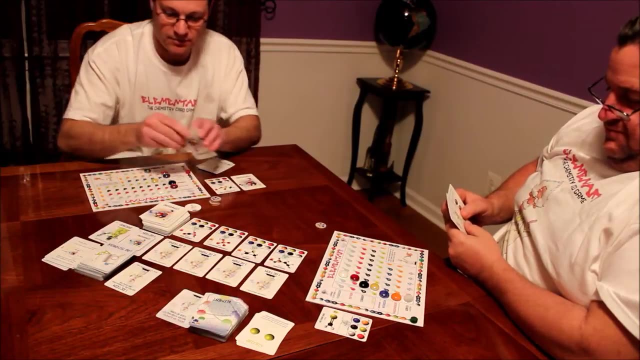 lab technique card. laboratory glassware. draw the top three compound cards, keep one and discard the others. I'm going to kind of get another bigger choice here. All right, I'm going to take this one over here. methane's sulfonic acid. put these into the discard. 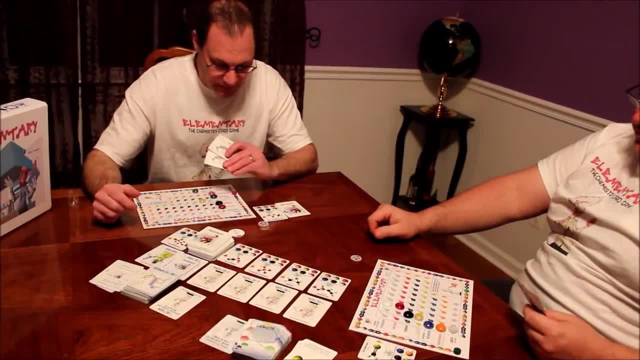 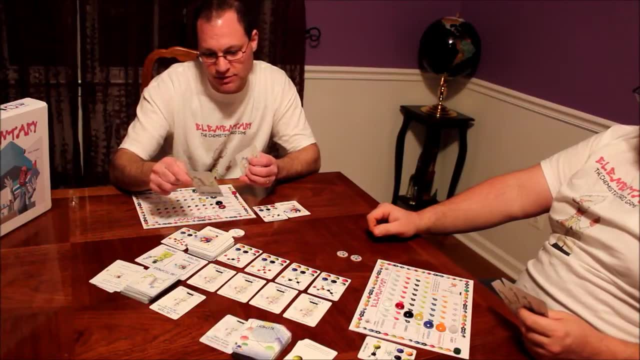 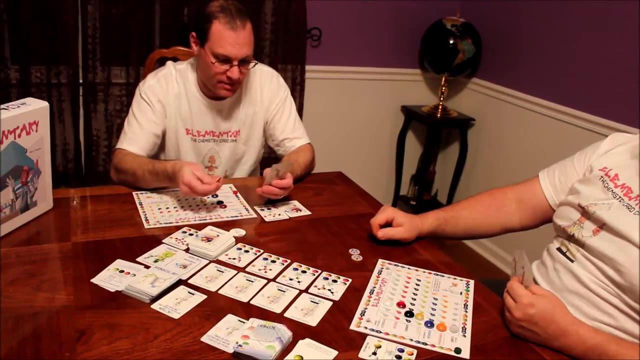 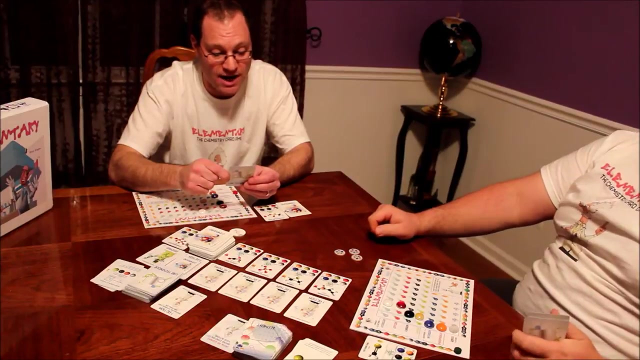 pile. All right, Four more actions. Okay, Play one more action: spontaneous fission. Swap this card for any one common element. I will take a hydrogen For my third action. I'm going to play this card. It's a dual action card. Select an opponent. deduct one common element. 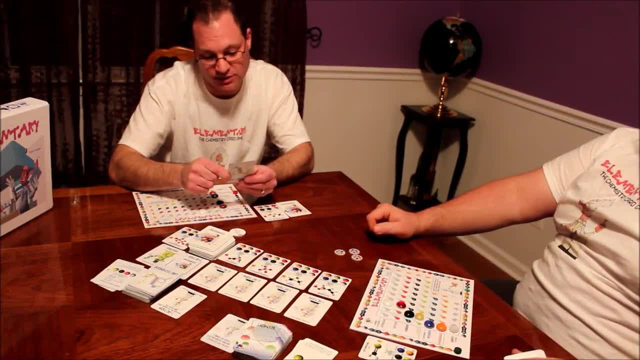 from their lab and add it to mine, Or I can use it to cancel a lab technique card played against me And then both cards are gone. Okay, So I'm going to play this against you If you have this radioactive man symbol here. 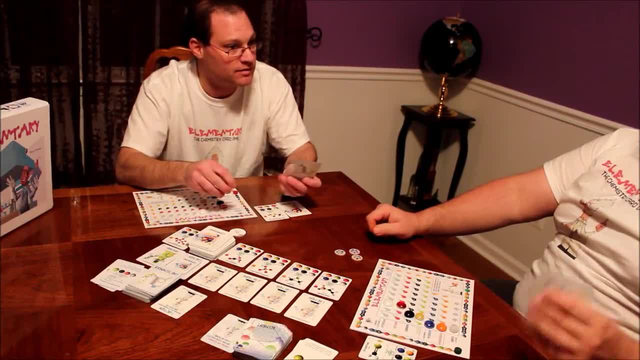 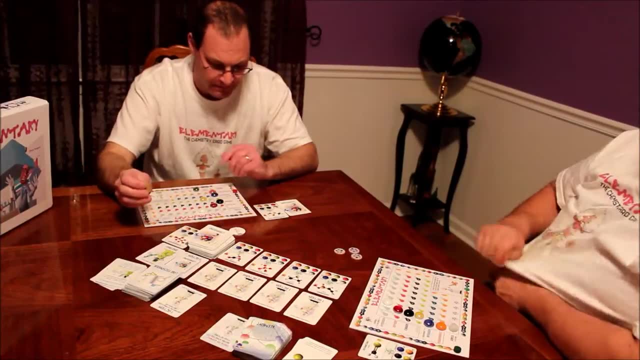 you'll be able to block me taking a common element from you And since I don't have it, I'm going to have to allow him to take it. So I'll remove one oxygen from him and he gets lost. That's what I'm taking. I'm taking the oxygen. Okay, I have two more actions I'm going to 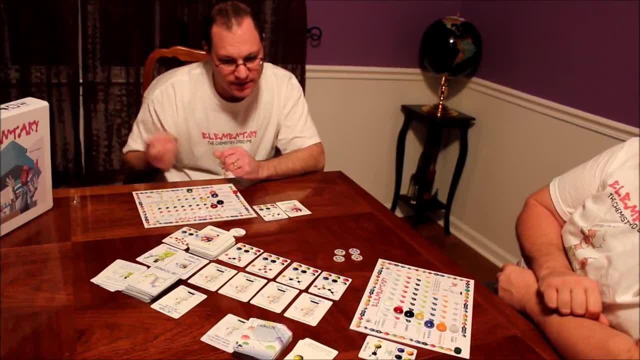 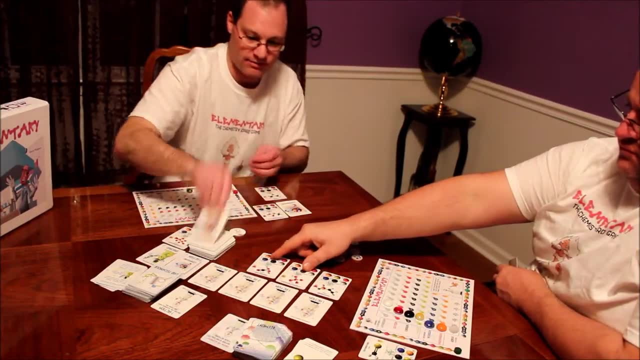 play one action and I'm going to buy one bond And I'm going to play another action and I'm going to take another compound from the marketplace. slide these down. That was a one action card, Mm-hmm, And pass my turn. 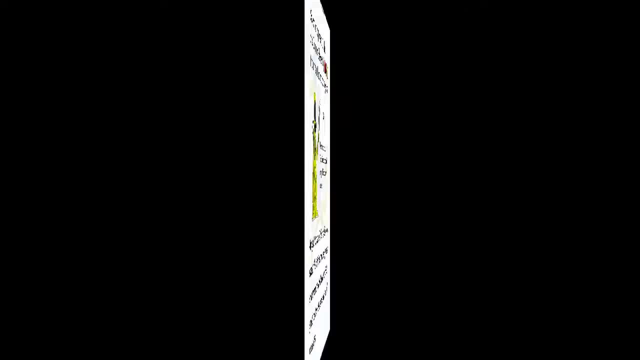 Okay, So I'm going to look at my cards. What I'm going to do is take some lab technique cards. There you go, So I'm going to always take my element card. I got a nitrogen, One of the uncommon ones, Those are hard to get. I'm going to look at my cards and see what. 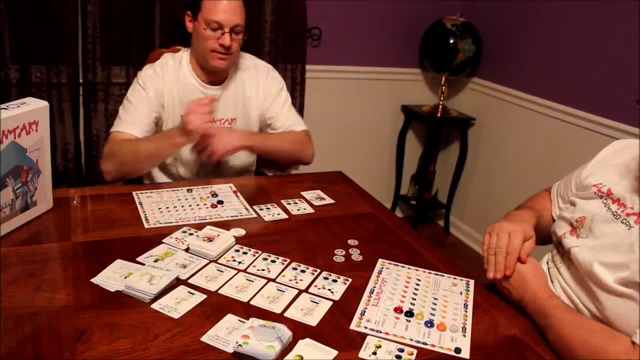 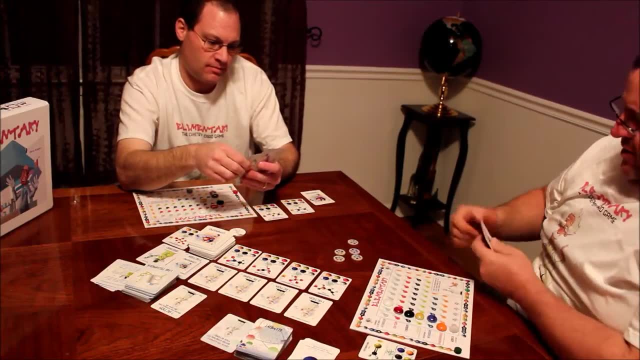 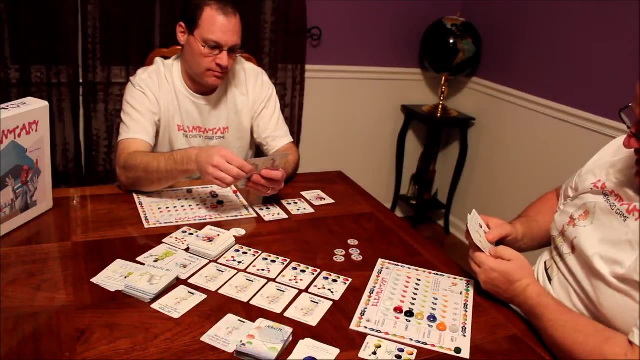 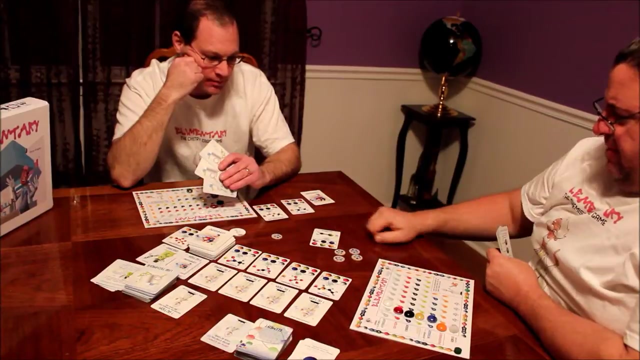 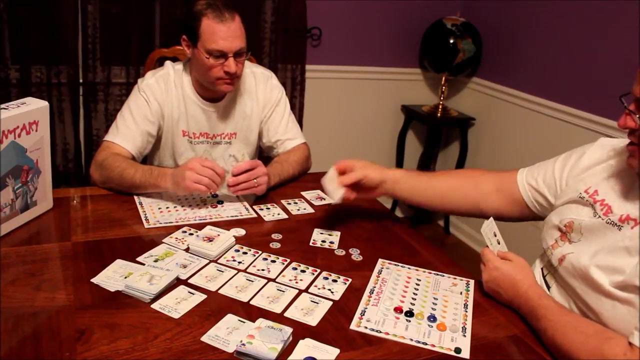 I want to do So the first thing I'm going to do is I am going to actually play one of my compounds. So I'm going to play this compound, But I'm going to look and say, wait, I have no bonds, But I can play an action to play one of my lab techniques. It's called magnetic. 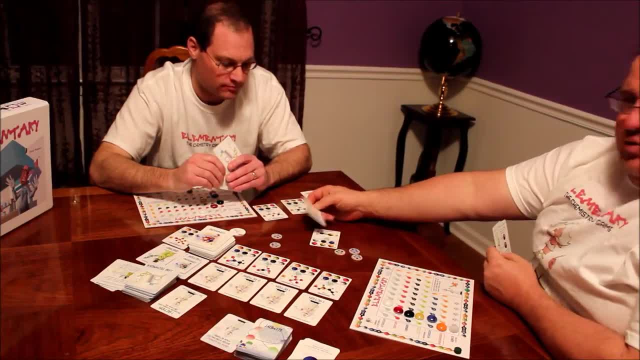 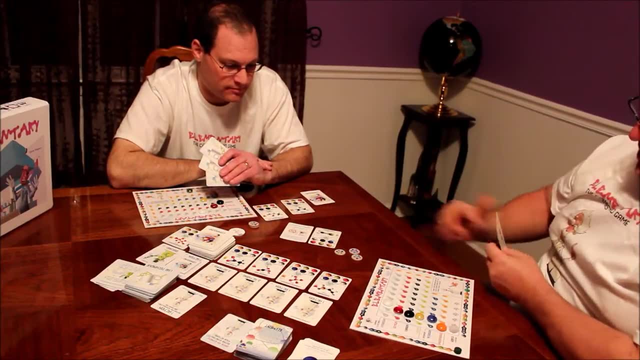 stir, And this allows me not to use any bonds when finishing a compound. So normally I would have to have two, But since I've played that, I don't need to spend the cost of the bonds, So all I've got to do is spend my two nitrogen One, two. 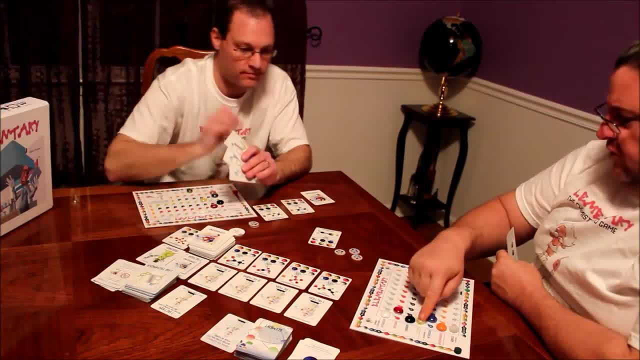 Okay, I'll spend my one carbon and one sulfur, And since I've played that, I don't need to spend the cost of the bonds. And since I don't need that, so then I will finish this compound. I will score the points. 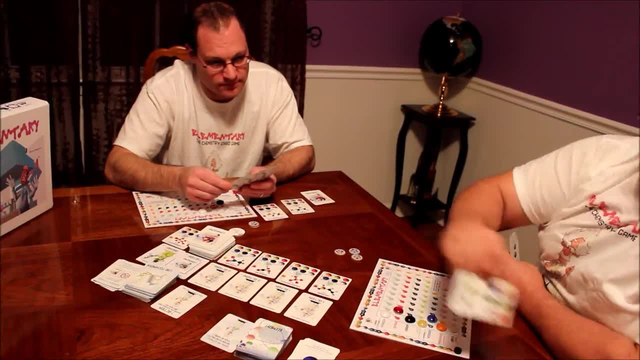 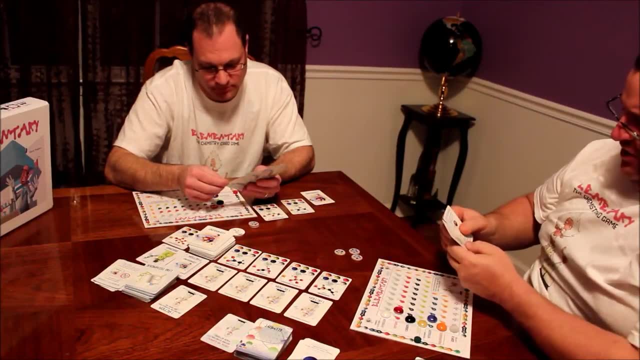 up in the upper right And that will give me five points And you know, yellow glassware. So that's later on for score And you'll see that I'll score my five points. I still have three actions. I'll look at my cards and say, okay, I'm going to spend an action, I'm going 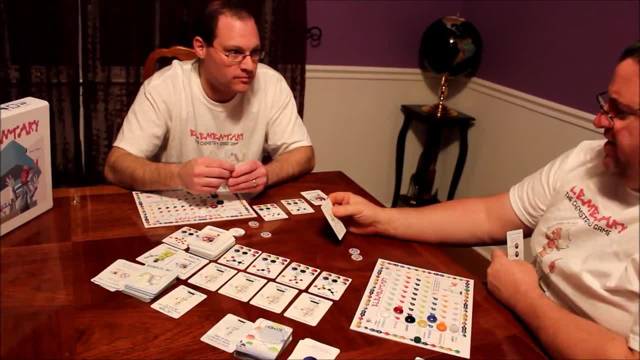 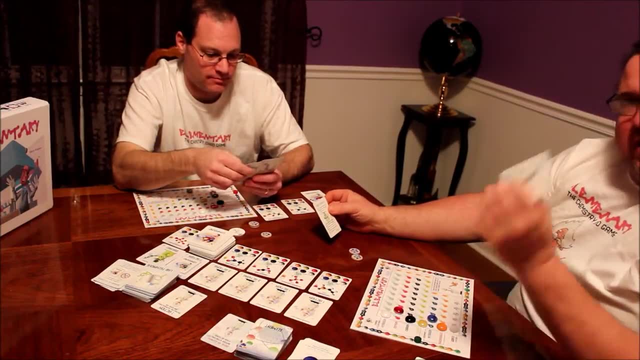 to play a card, a lab technique called bond enthalpy. This allows me to select an opponent, which is him, And he has to deduct two bonds- Two bonds from the lab And I'll get to add one bond to my lab. So I'm going to play this. 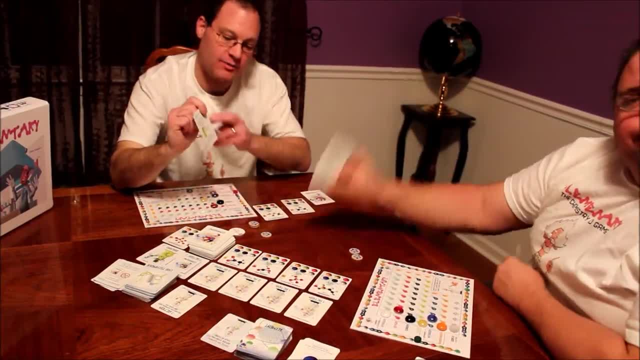 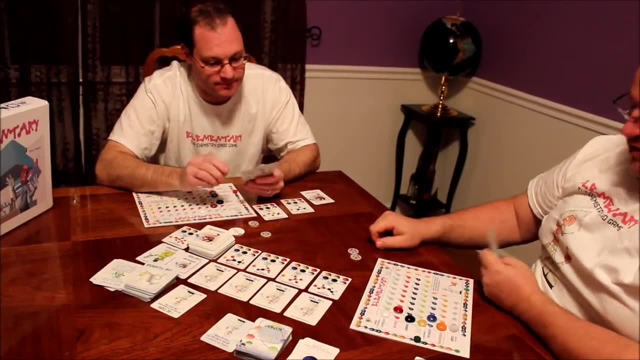 on him now whether he has a card. I am going to block that with my radioactive Block me. So basically those two cards go into the trash, So I save my curses. And then I don't get my new lab technique card until the end of my turn. So I still 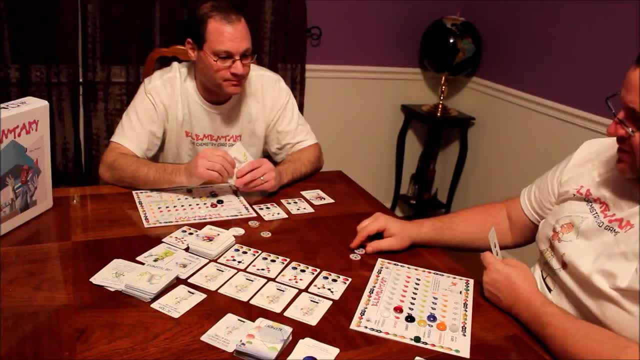 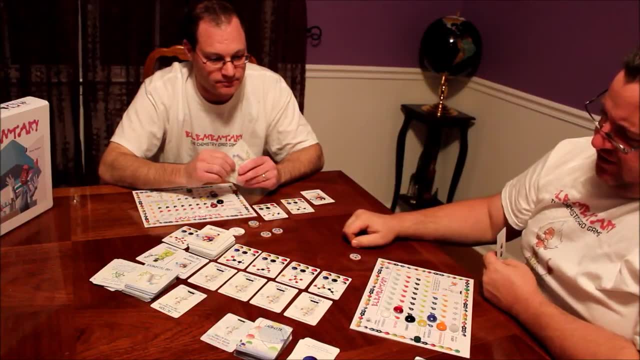 now only have two Right, So I still have two actions left. So I'm going to have to get some stuff I've got to work on, So I'm going to spend one action. I'm going to take hydrogen phosphate out of the compound. 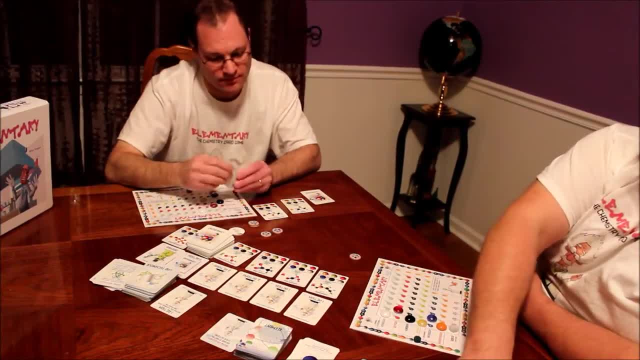 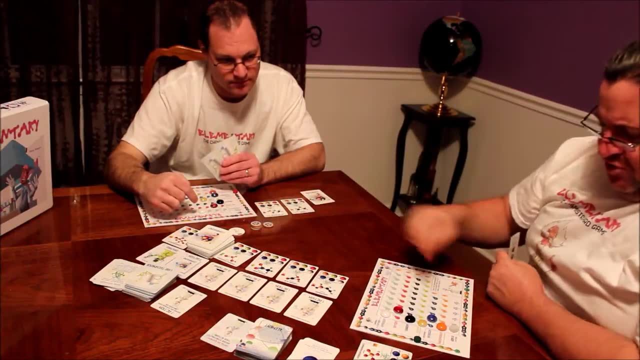 marketplace Put it there, I'm going to keep the score one off to the side. So I've got something to work on And I've got one more card And I'm just going to go. I'll purchase one bond, I'll move the bond up one on my laboratory And that is my turn. I always 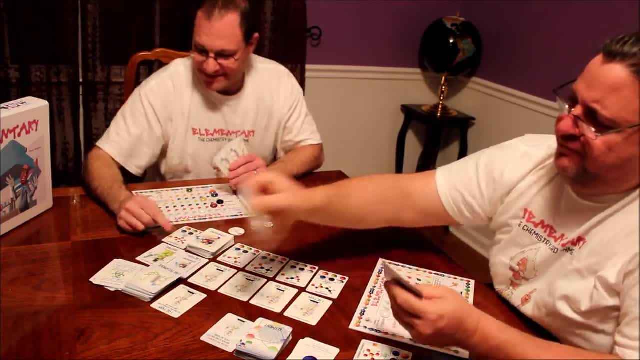 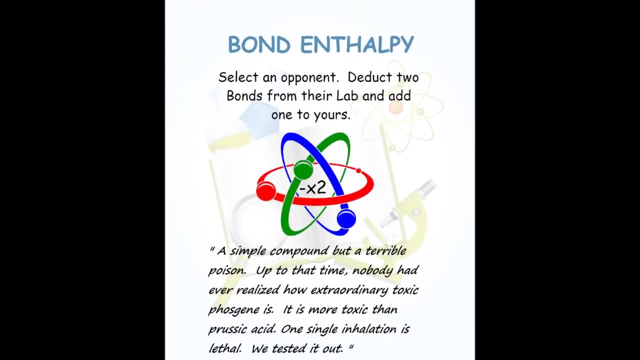 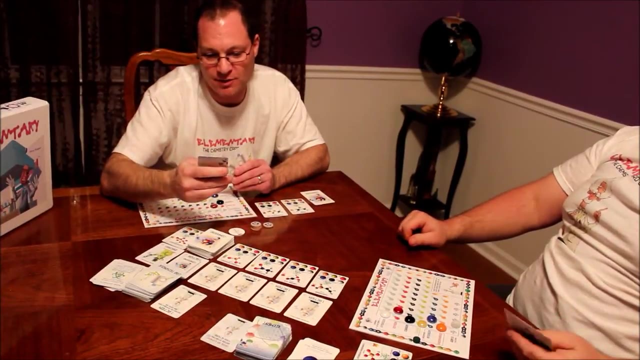 got to get my lab technique cards And I've got my. I go up to three, And then now it's his turn. Endful plea of combustion, Lab fire. All players deduct one common element from their lab. Active player's choice. 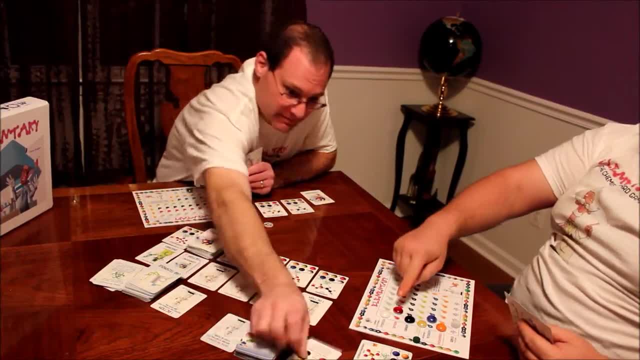 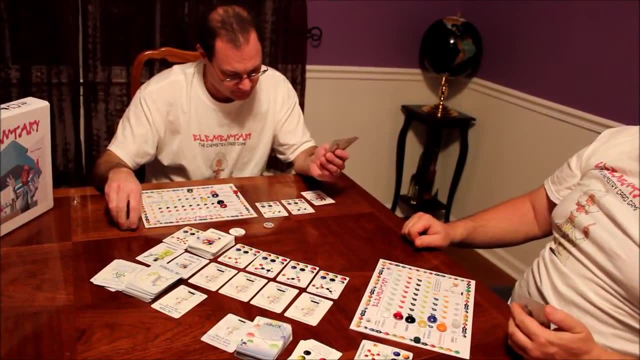 So everybody's going to lose an oxygen, Right? So there's nothing I can do. Even if I had that radioactive guy card, I'm not able to block it. So it happens to everyone. So it's tough luck in the science world. 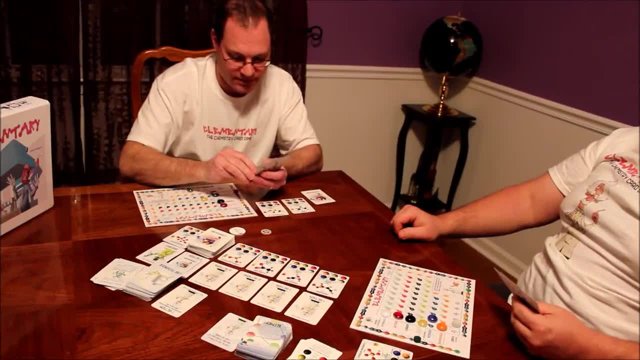 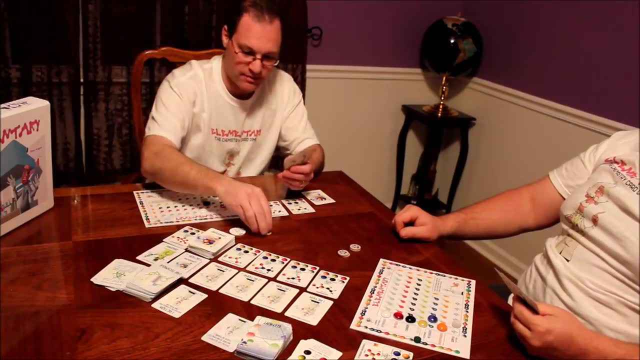 I have some limited options here, but I'm going to go with the radioactive. There's limited options here, but I'm going to try this. I'm going to spend two actions to buy one carbon. I'm going to spend another two to buy a second carbon. And my last action: 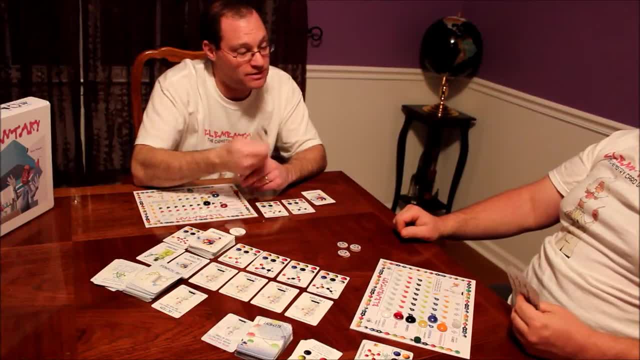 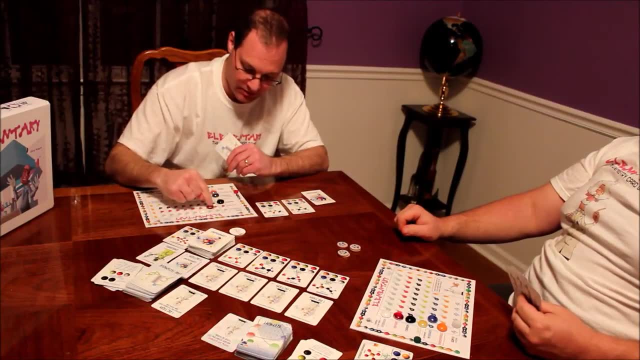 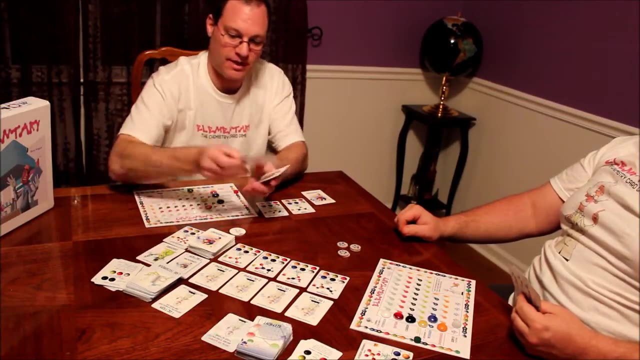 I will play covalent bond, swap two carbons for any combination of three: hydrogen, oxygen and sulfur. So I will remove those two carbons, I will take two oxygen And I will take one hydrogen, And that will take my lab techniques up to three. 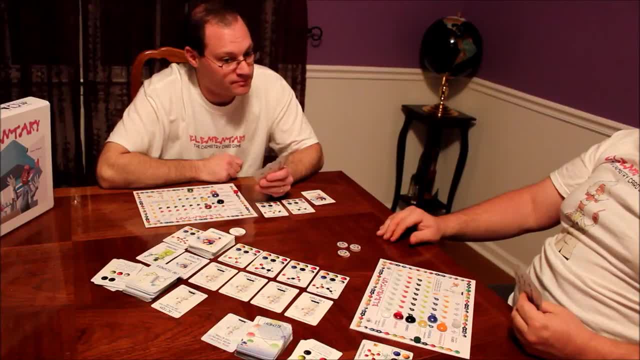 Okay, And it's your best turn. So what we'll do is we'll play a couple rounds and we'll get down to the end- kind of toward the end- score. So we'll continue playing and then we'll come back when we're going. 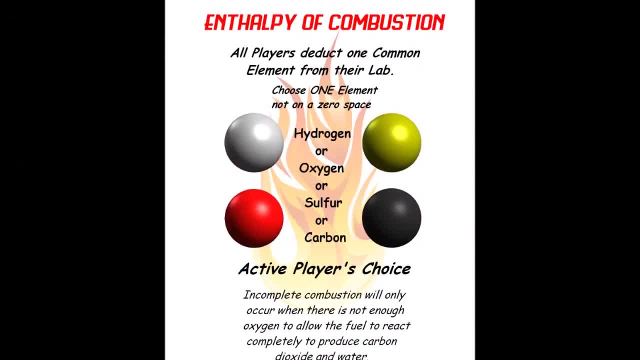 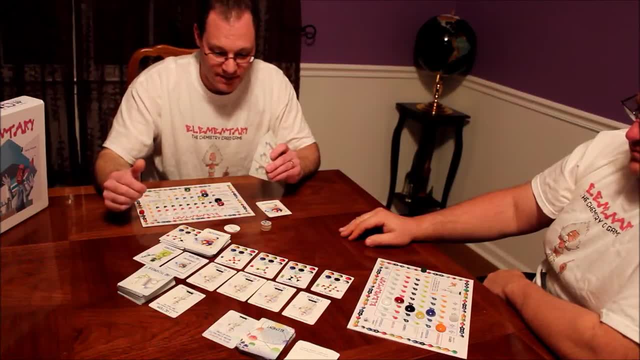 to kind of score at the end. All right, We're back. We're going to finish up this game. Yep, We're getting close. We played a couple rounds. We're getting to the end. I got 38.. I think he's got. 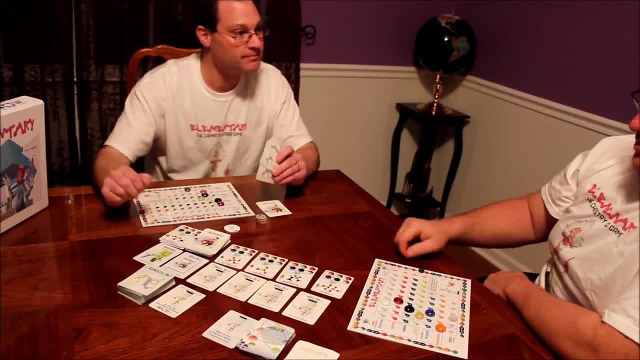 I got 36 points. All right, All right. Well, you got the mark, so let's go. All right, Let's draw an element, All right? Uh-oh, That's not good. I got two hydrogen here. 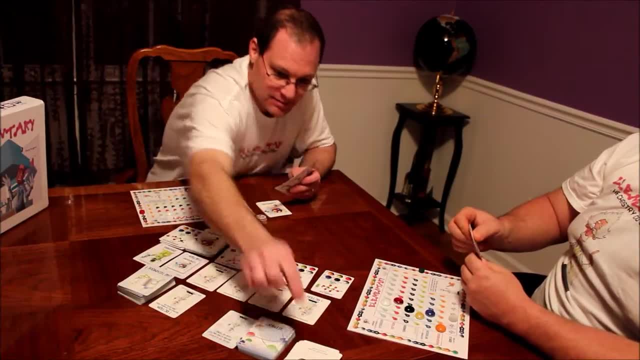 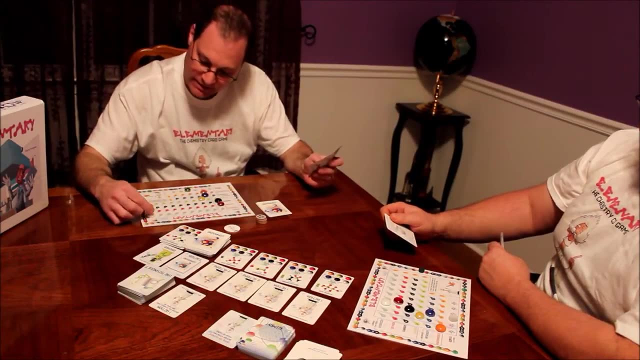 Ah, And I'm already at seven. So this is a problem. I go to eight and then I'm going to deduct one compound point for every element gain that I can't store in my lab. So I'm stuck at eight and I lose one compound point because I went one over. 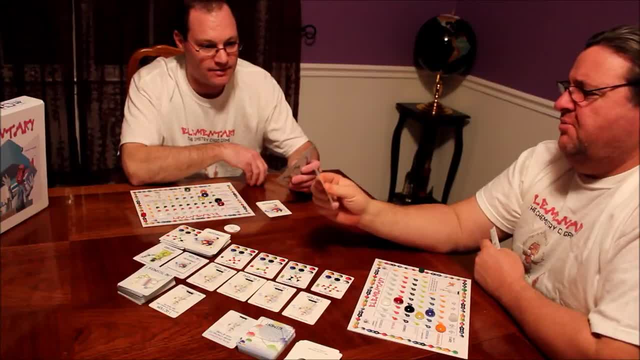 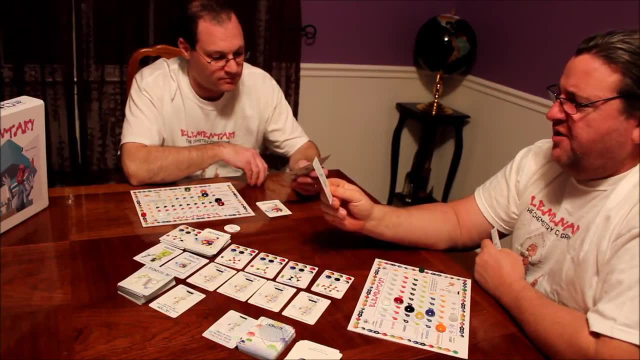 Yeah Well, one man's pain is one of the man's pleasure, because I'm going to play this Faraday constant. What that allows me to do is, when he drew that element card, when my opponent draws the element card, I can play the card and add one of those drawn elements. 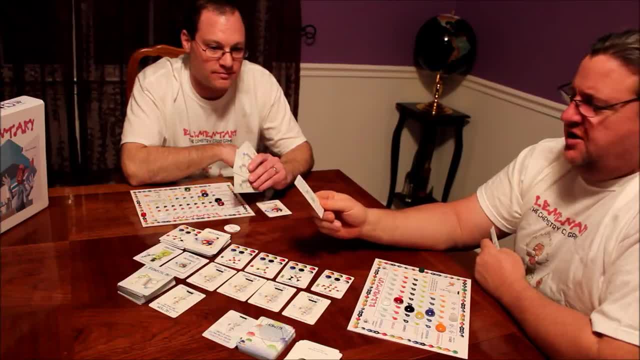 So I can add one of those drawn elements to my lab. So that's another way You can sneak your way in and get some. Now I can't play this when there's a specific card, entropy or enthalpy- So I'll be able to. 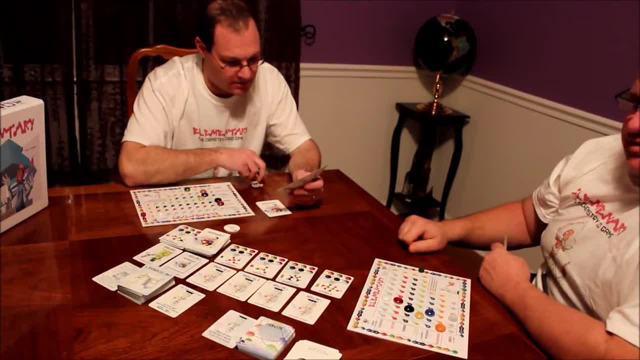 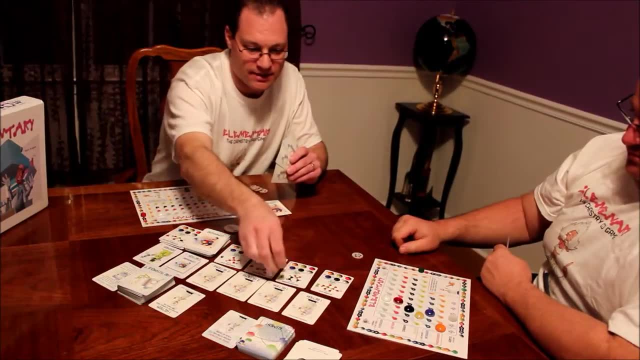 One hydrogen, So I'll be able to get one hydrogen. So there, All right, Let's see what I can do with my five actions. Keep blowing up. I am going to spend one action in the marketplace and I am going to purchase vinyl sulfonamide. 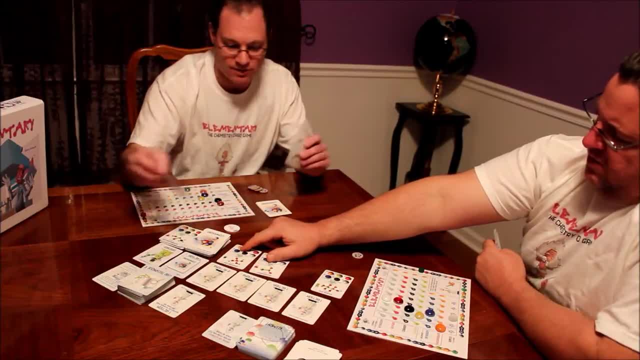 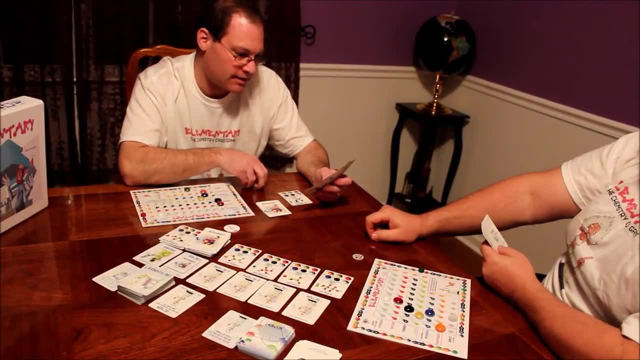 the 14-point green glassware symbol. All right, So everything slides down and gets progressively cheaper. Mm-hmm. Okay, Let's see if I can do some damage here. I am going to play this card on you. It's radioactive tracer. 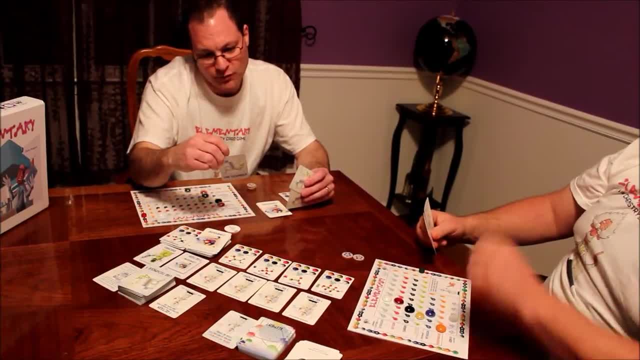 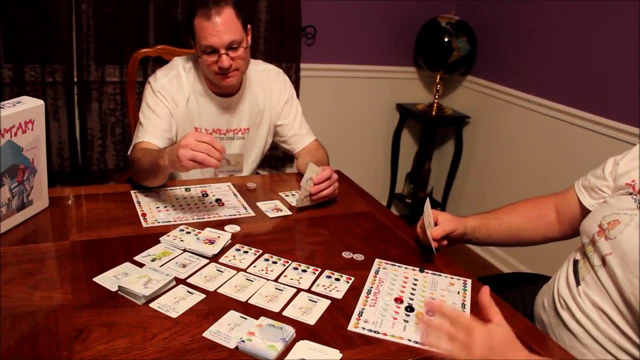 All right, I can't block that. This is going to force you to complete this small compound, hydroxide ion, before you can complete any other compounds, Right? So if I had some compounds out here I was working on, he's going to play that. 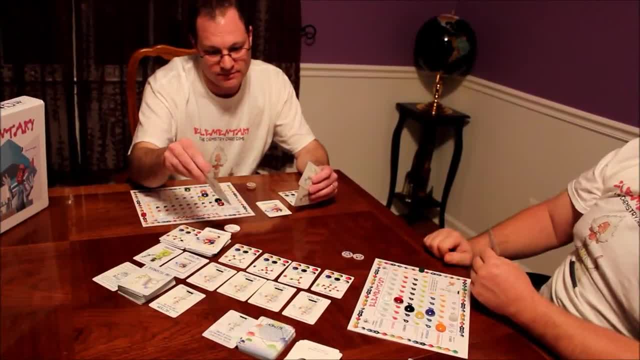 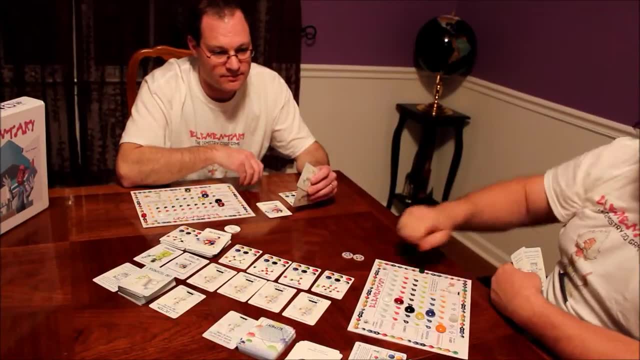 on me and I'll not be able, Since I don't have the little radioactive man to block him. I can't block him. He plays it on me, He plays it on me and I have to work on this little tiny radioactive tracer, to kind. 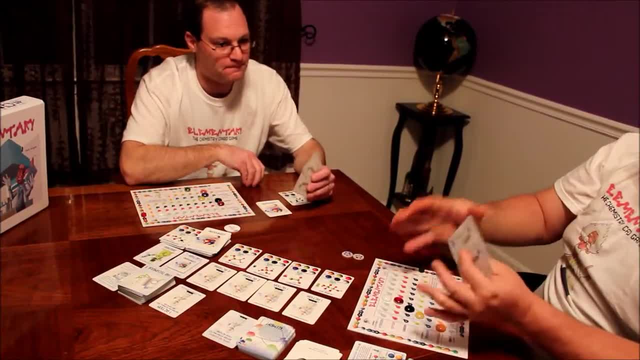 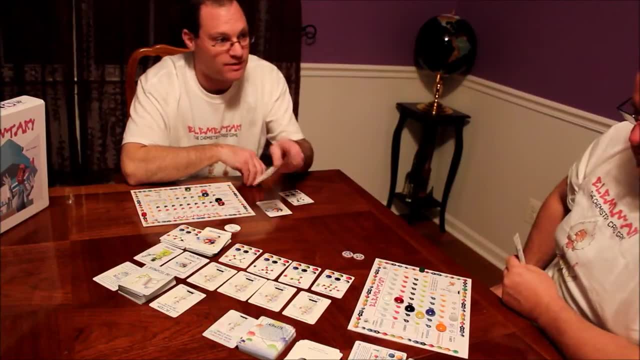 of get rid of it. So I can't put any more resources toward any other compounds until I finish that. So it's kind of slowing me down a little bit, And that's still worth three points if you do finish it, Right, Right. 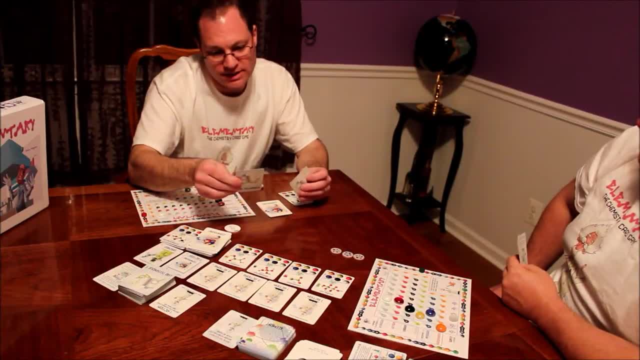 Okay. So now I'm going to play dynamic equilibrium. Select an opponent. Take one random lab technique card, All right, And I can play it immediately at no action cost. All right, Let me shuffle these up a little bit, All right. 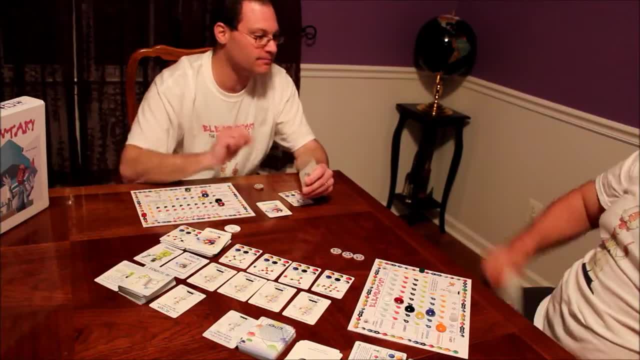 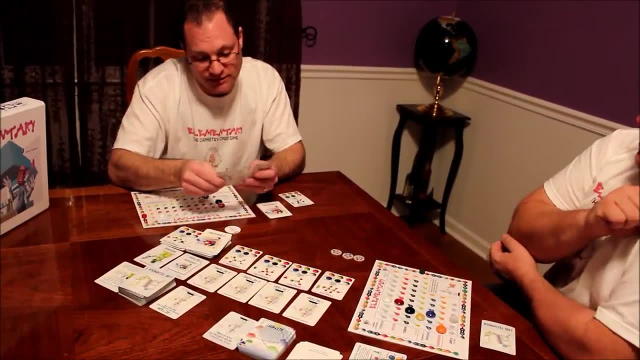 I can't play it, I have to discard it, Right. So shuffle, shuffle this up. I'll try this one. Okay, Single replacement: I can play this immediately for no action. Take the top three element cards, use one and place the other two back in any order. 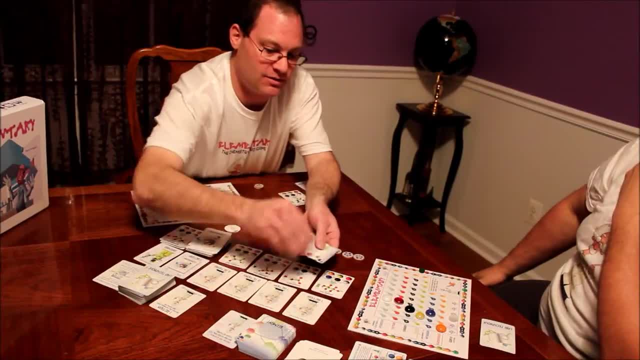 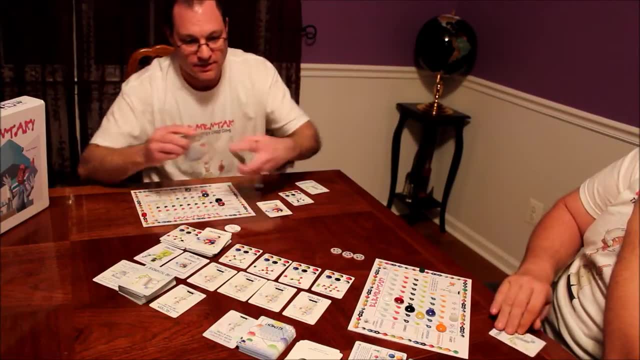 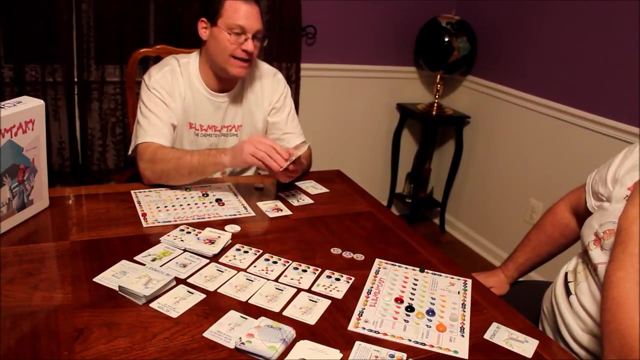 Okay, Let's see what I get. One, two, three. Okay, This is pretty simple here. Put them back like that, And I'm going to take entropy. It's a add any two elements, So I'm going to take that. 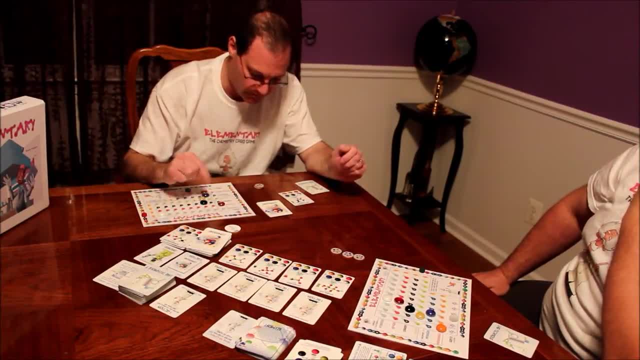 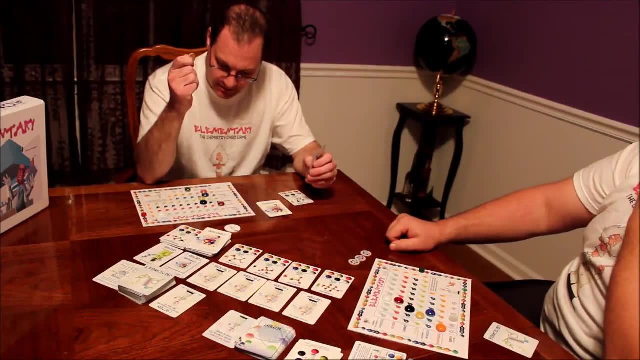 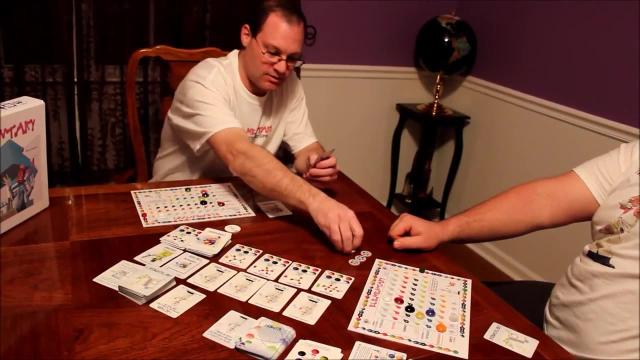 And let's see what I end here. I'm going to take two carbons, One, two. Let's see what else I have here. I am going to looks like I'm going to need to purchase a bond. I'm going to take these two, but I am going to purchase one oxygen. 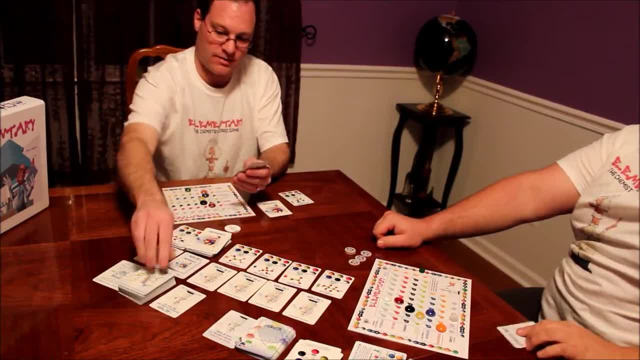 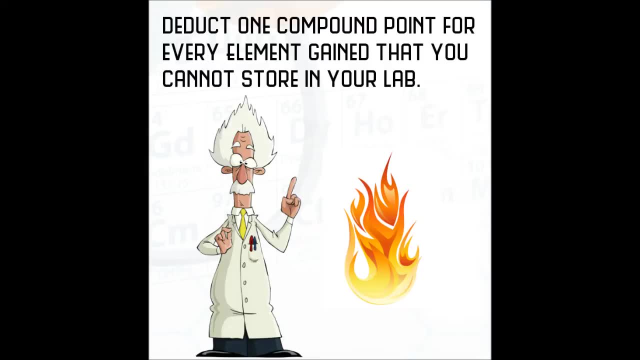 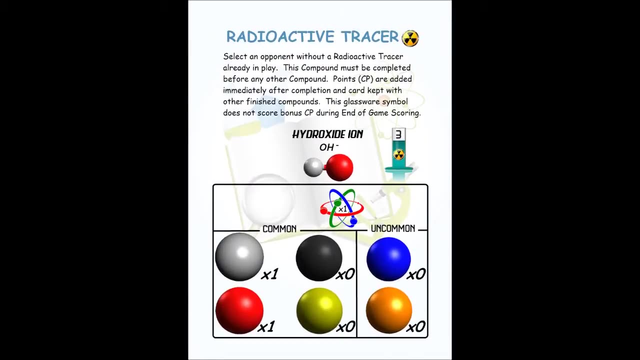 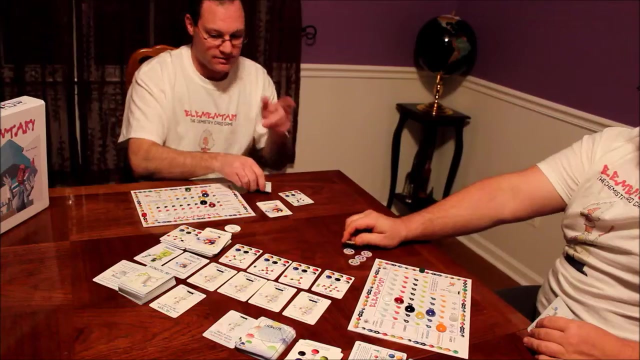 So you can buy any common element with two elements. Okay, I'm going to buy a common element with two actions. Two actions, I'm going to buy one. Yes, And I got my three cards Set to go, Okay. So, as always, as you probably know by now, you just draw an element, Okay. 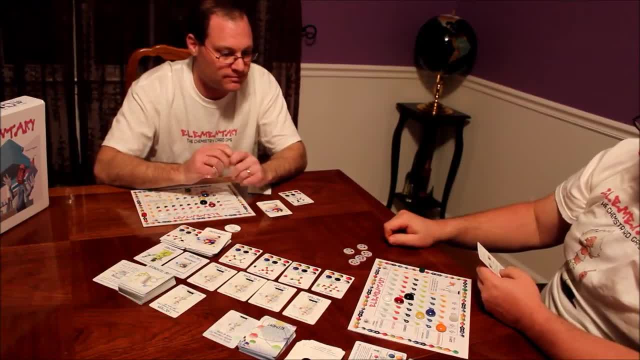 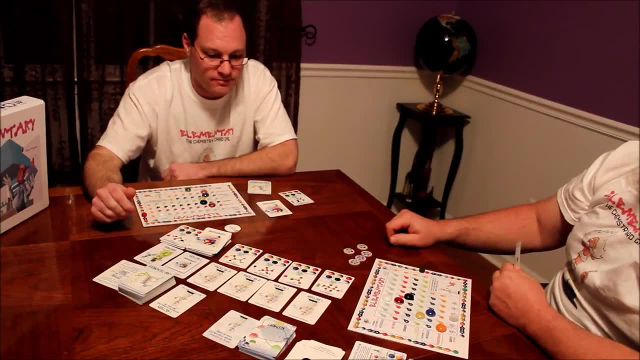 I'll grab two carbon. So one, two. All right, So I have my actions. So I'm going to look, I'm going to try to kind of work on that. I think I am going to spend an action. Then I'm going to play this card. I'm going 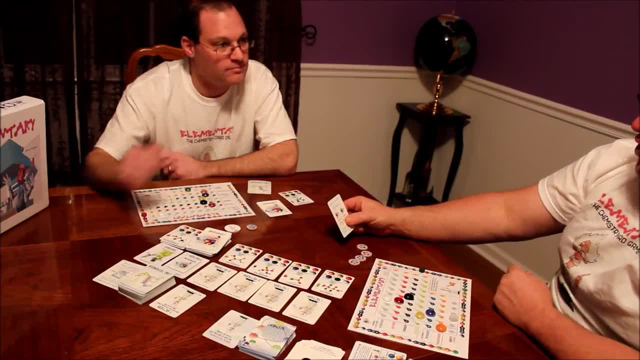 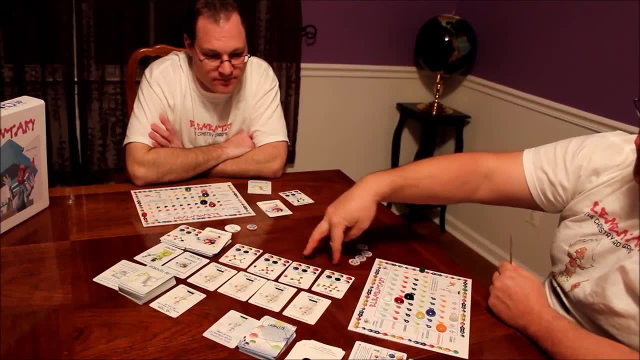 to play a neutralization reaction That's going to allow me to take two actions in the compound marketplace. So what I can do is I can either take one card from the two action area or I can take both of these cards. So I'm trying to end this game quick. I'm going. 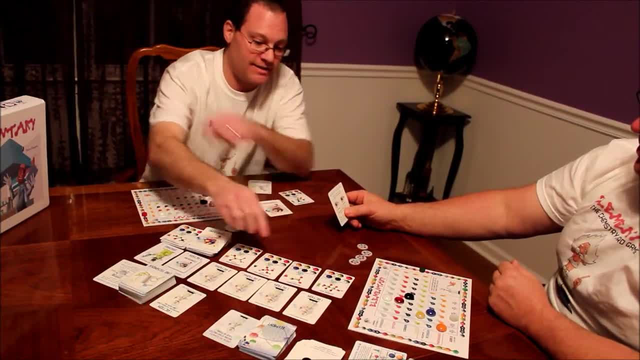 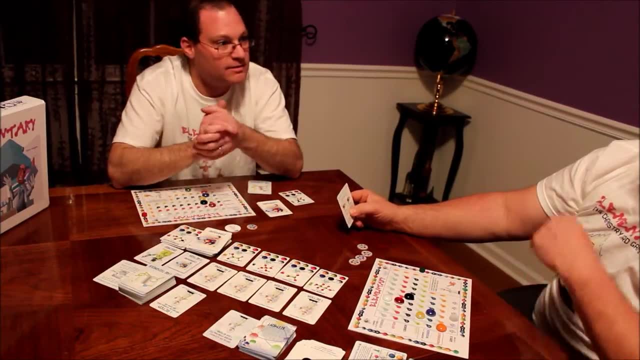 to try to get something. That's another point. You could take a one action card and they slide down immediately. You'll be able to take another one as well. Okay, From the two, They slide immediately. So they slide immediately. Well, that's another thing I remember. They slide immediately. 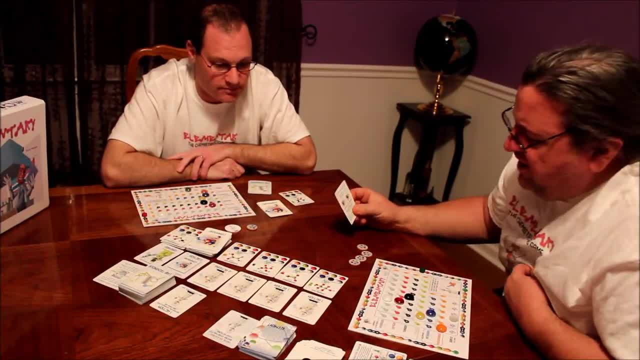 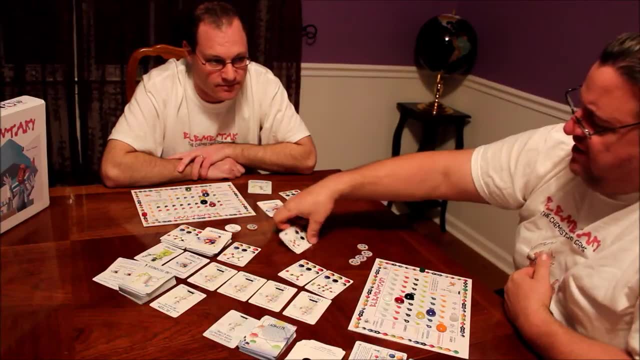 What I'm going to do. anyway, I'm just going to see if I'll look at an easy one that I could probably do where it's doable, And I will play that and I will try to get this one. So, since it's a two action card, I can take the one for free, But the only problem. 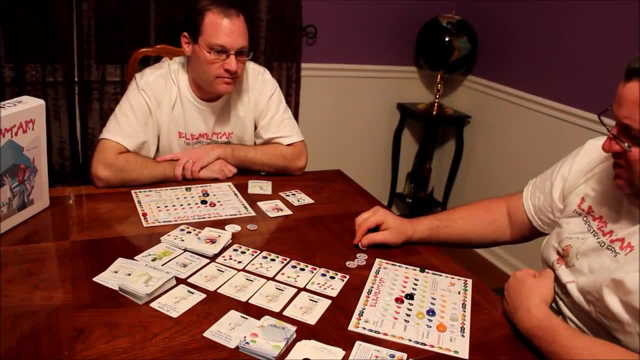 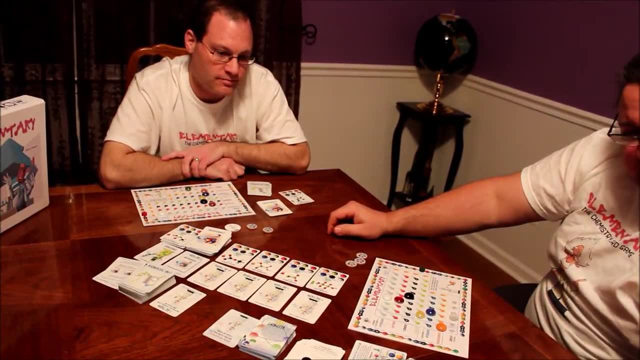 is. I'm going to have to work on that And that's what I think I'm going to do. So I'm going to spend my one action. So, as I said, I can't put any of my elements toward finishing this phosphoric acid. So I'm going to try to get rid of that radioactive tracer And 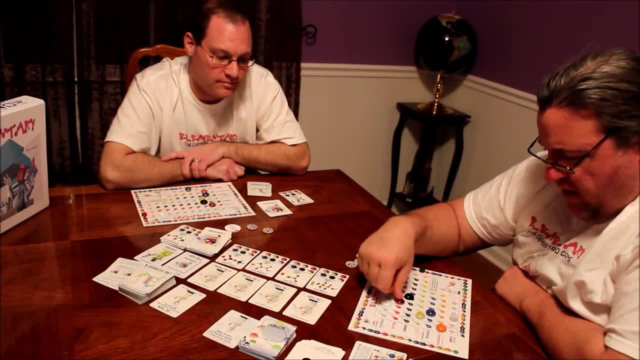 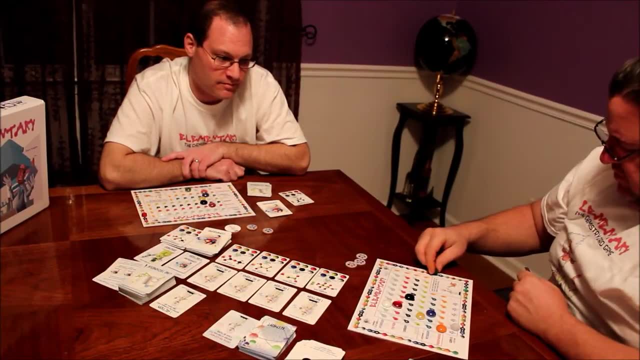 I'll spend my one hydrogen, I'll spend one oxygen And I'll spend one bond. So it took me down a little bit, So I'll have I'll go up three points, So one, two, three. So I'm. 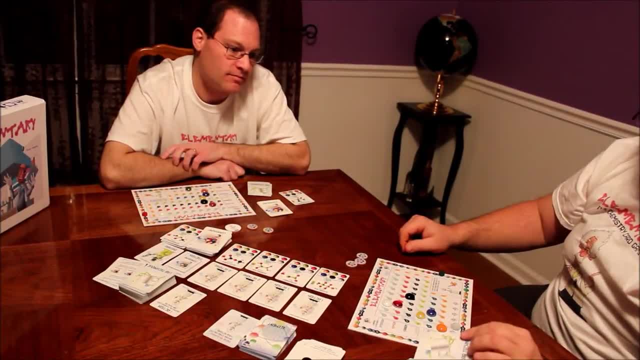 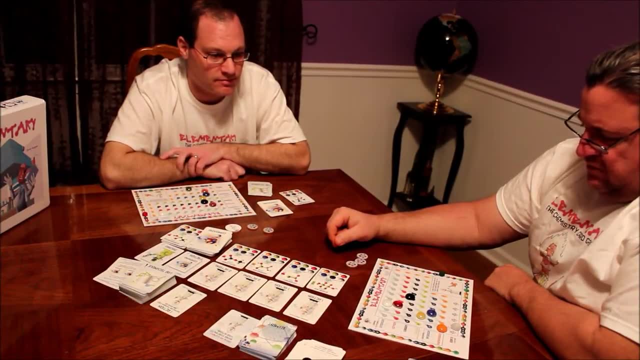 going to keep this, But at the end, the glass word, well, yep, the end of the game score and we'll show you. All right, So I have three points, All right? No, I've got this. What am I going to work on? 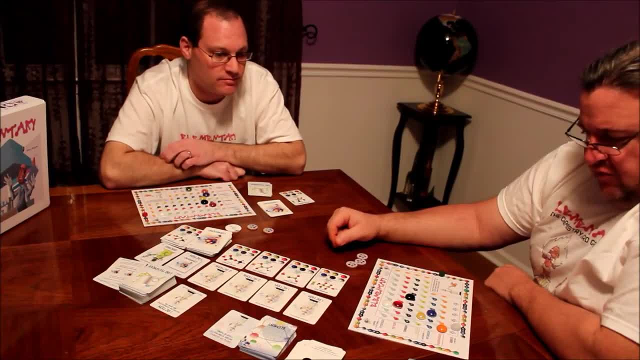 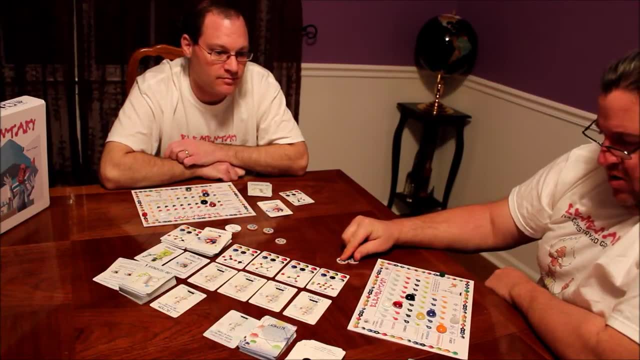 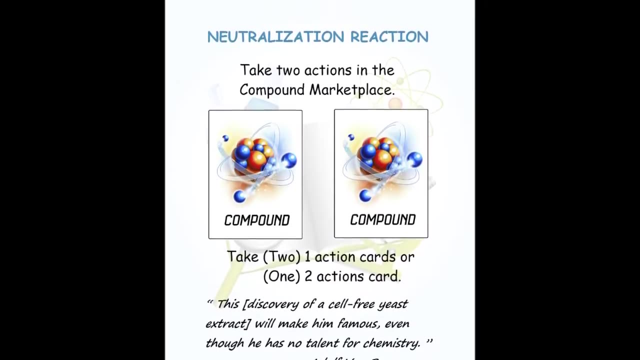 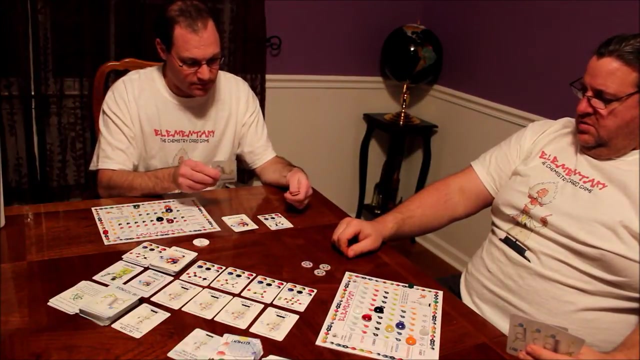 So I'm working on that. What I can do is I can buy a bond, which I think I'm going to need, And then, for these last two actions, I am going to buy a hydrogen. All right, I am going to play an action and finish this compound, And I'm going to do it with a unimolecular. 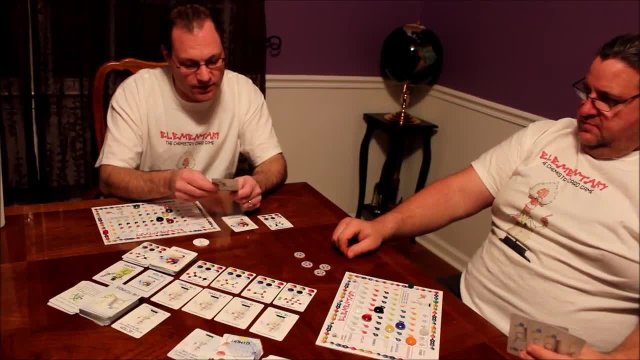 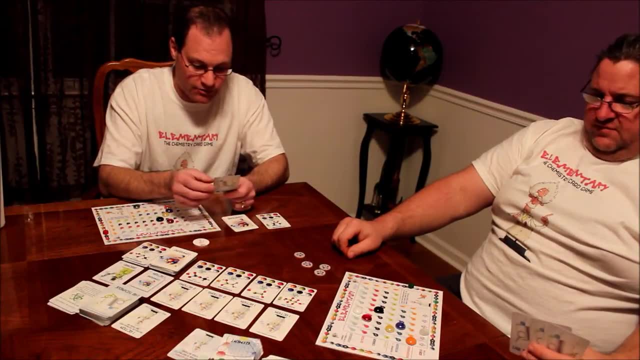 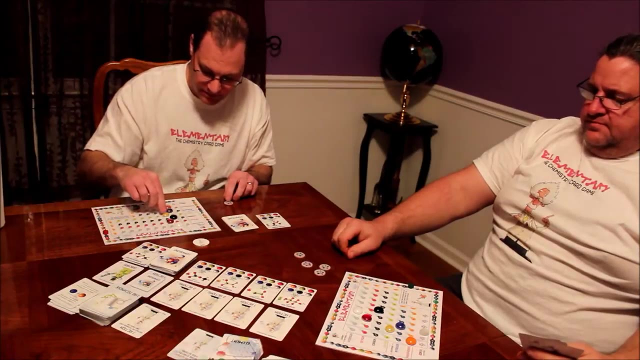 reaction To complete a compound. any one uncommon element is no longer required, So I'm going to not worry about the. Let's go with the cost of the nitrogen there, Mm-hmm, All right. So one, two, three, four, five. I have two carbons, sulfur, two oxygen, four. bonds: 14 points. So how much was that? Thirty-eight, Forty-eight, Fifty-two, Okay, Oh, and actually I was down one because I lost one from the fire, Right? So I'm at fifty-one, Mm-hmm. 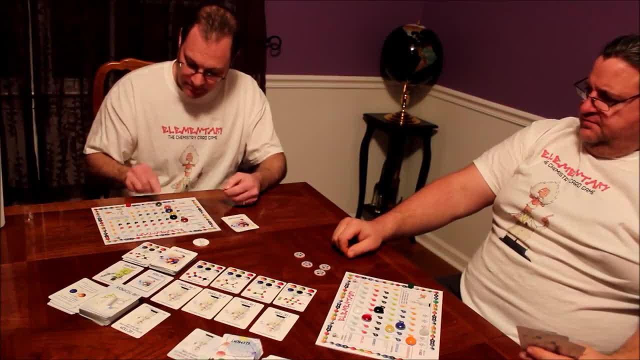 And I'll buy a bond. Mm-hmm, And I finished. but I'm the first player, which means you still get one more turn. I've got one extra, So everyone's going to have an extra. So if you land on, you either. 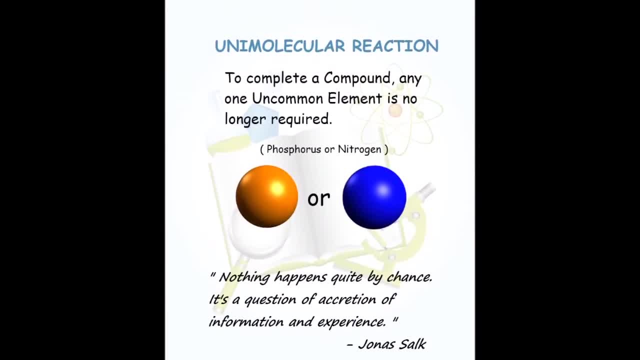 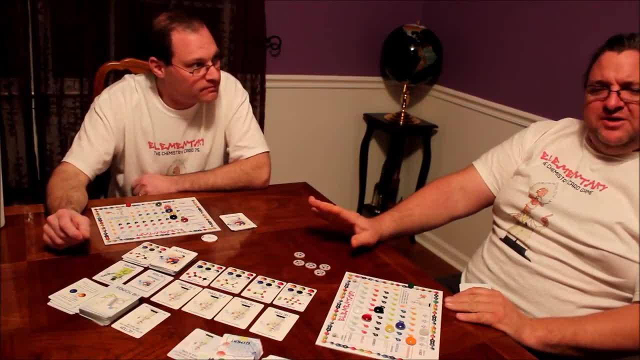 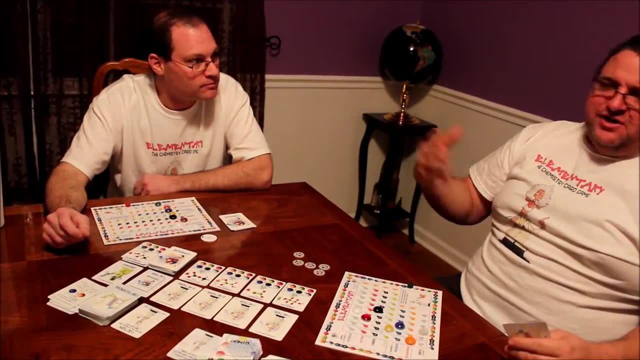 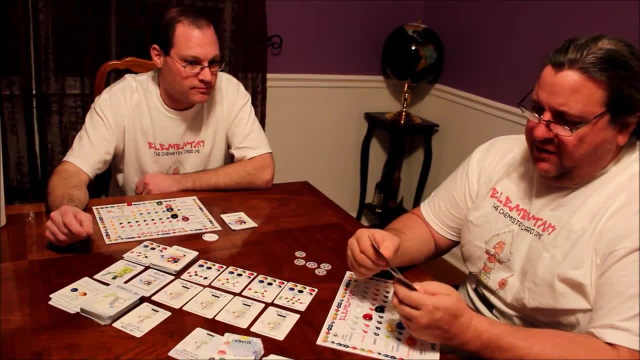 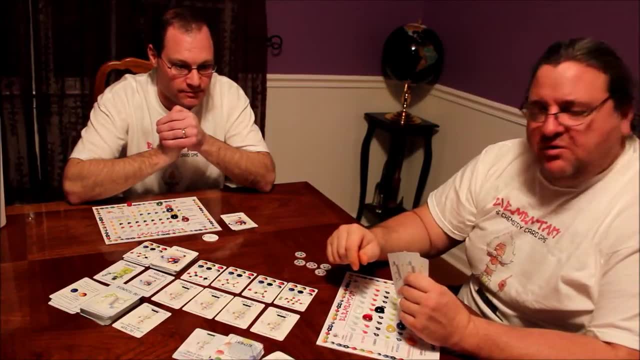 get an equal number of turns. Let's see if I can make sort of a comeback here. I'll figure this out, Okay? So, as always, I draw my element. Okay, I'm going to go blow. The lamp blows up, So I'm going to choose. 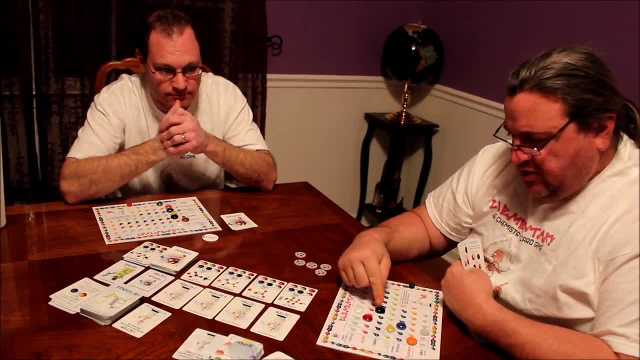 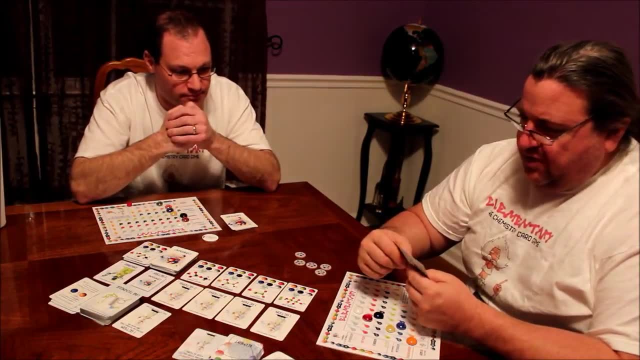 what elements to lose. So actually, what I could do is I am going to lose a carbon. I think I'll lose a carbon. All right, So that wasn't good. All right, I know it's going to be a long way, so for my first action, I'll spend my one action. 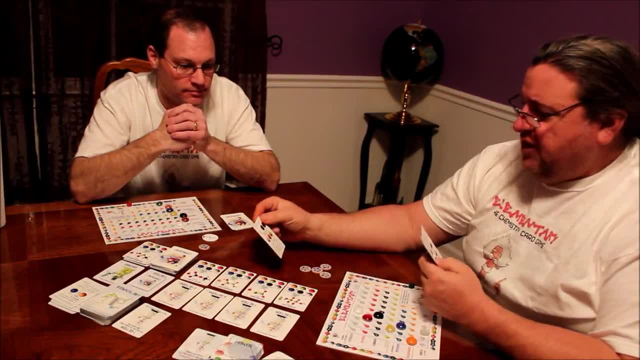 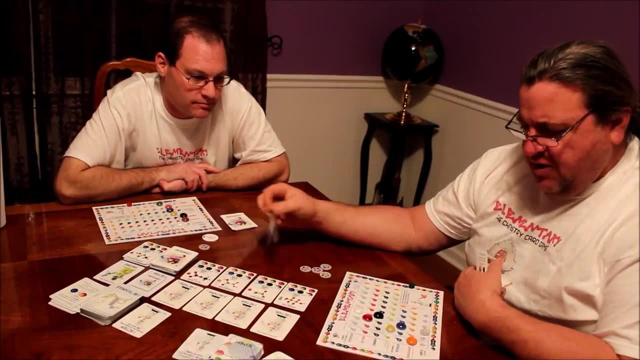 give it over to him. I'll play this covalent bond. this is going to allow me to swap two carbon for any combination for any three of either the hydrogen, either the oxygen or the sulfur. alright, so I will do that because I'm kind of eyeing something up over. 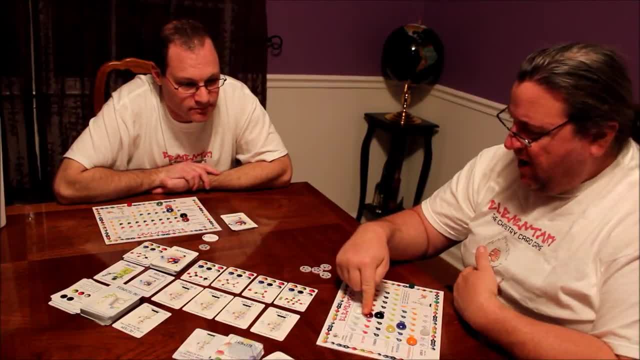 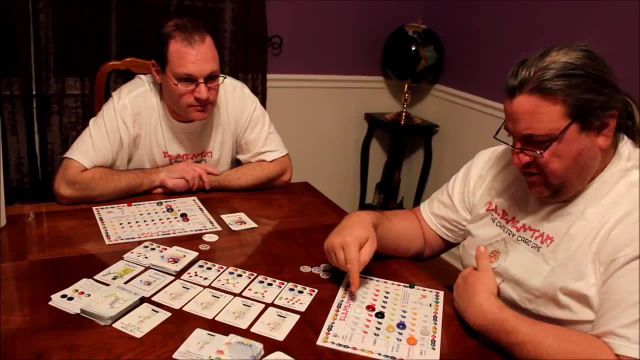 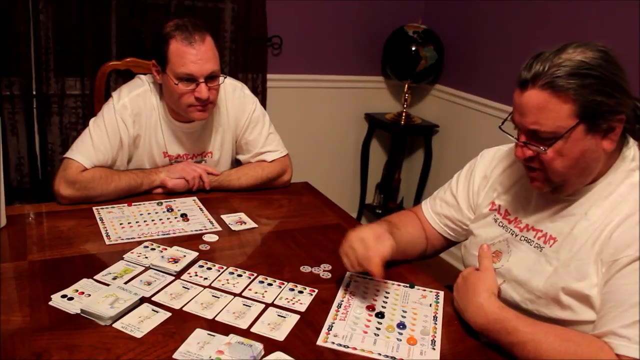 here so I can go. I'll go up one on my oxygen. I'll go up. I'll go up two on my oxygen actually and I'll just go up on actually. no, it's oxygen, right, so I'll go up one on my sulfur. 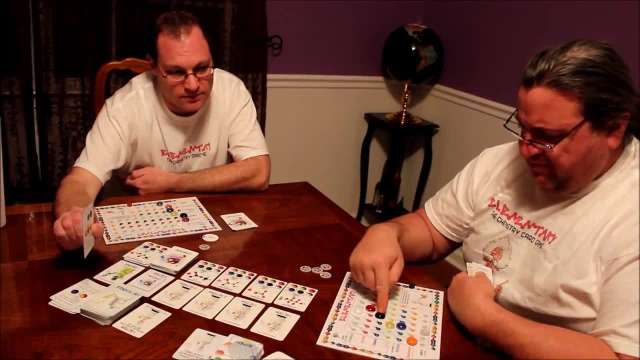 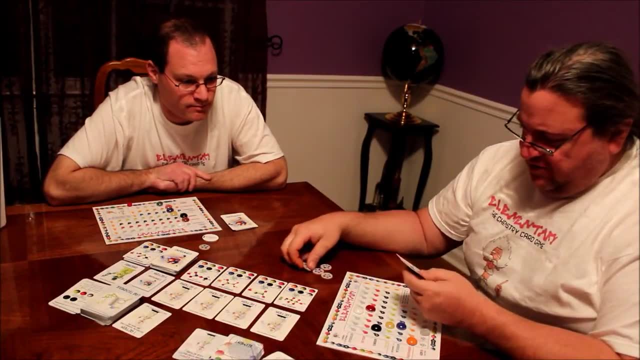 And drop down the carbons. I dropped down the carbons right, one and two, yep, so right down. so you always do that first. you always remember that. So my my, I'm going to do another action. I'm going to do so. I'm going to so, since I'm going, 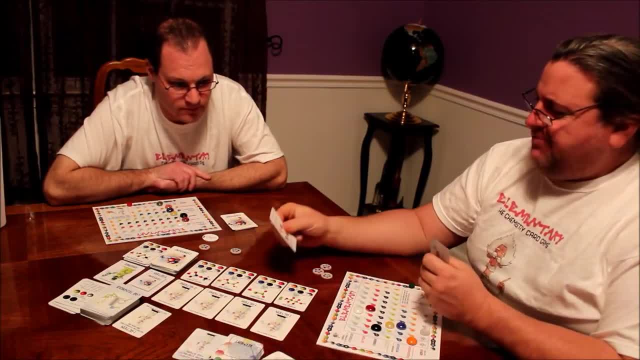 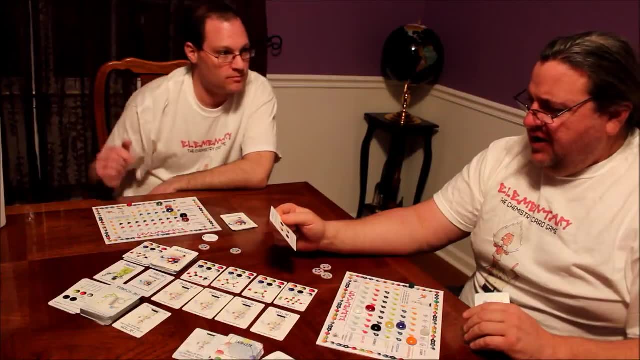 to need something over there. so I'm going to just pay this one action. I'll play this lab technique card. it's called synthesis. What this allows me to do is I can trade one of my uncommon item elements from an opponent and I can then yeah and then. so we're basically trading off. 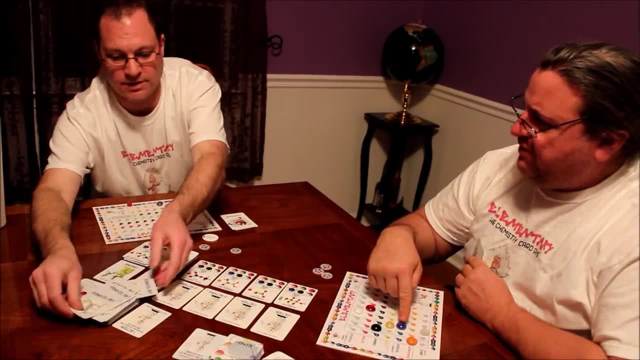 So I'm going to, I'm going to give him a nitrogen, I'm going to give him. You have to give him my three cards. Okay, there you go, Because if I could block this, if I got something which I didn't get, then you could block any. 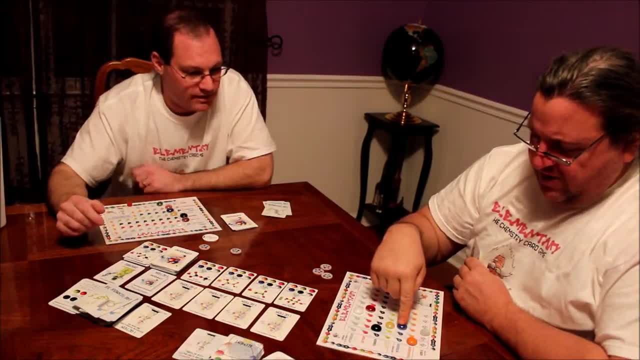 type of trade in the game as well. Right, exactly, So it's not as nice. There's nothing I can do to block that. So I'm going to give you a nitrogen and I want to take one of your phosphorus. 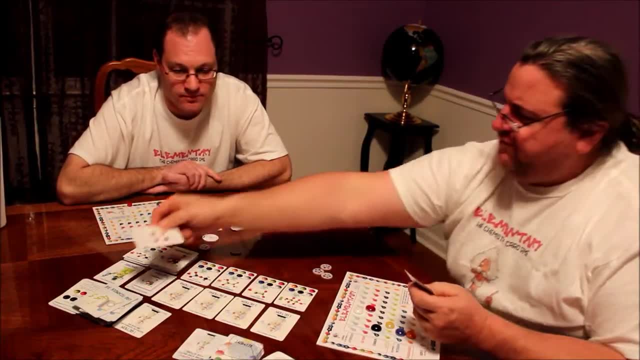 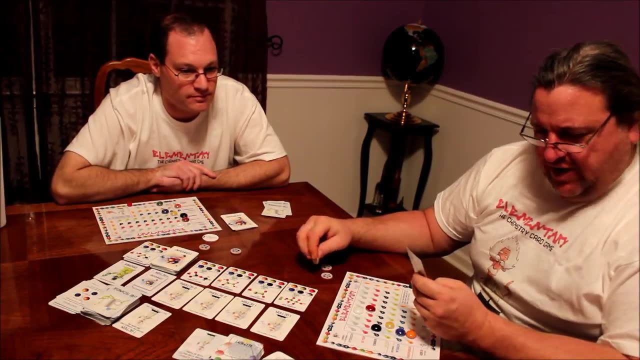 Okay, So I'll go up on phosphorus. so that's okay, I'm going to take that. I'm going to play it there, All right, Okay, so I'm going to try to complete this, hopefully get up here, so I'm going to play. 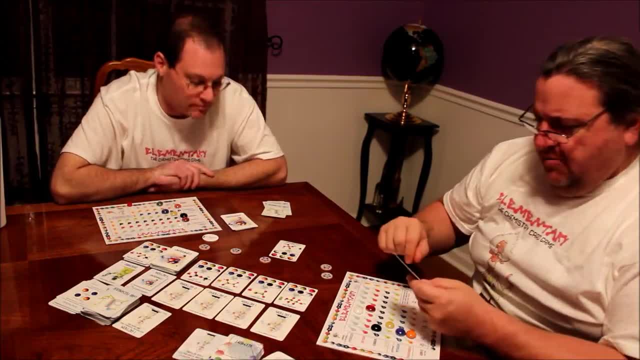 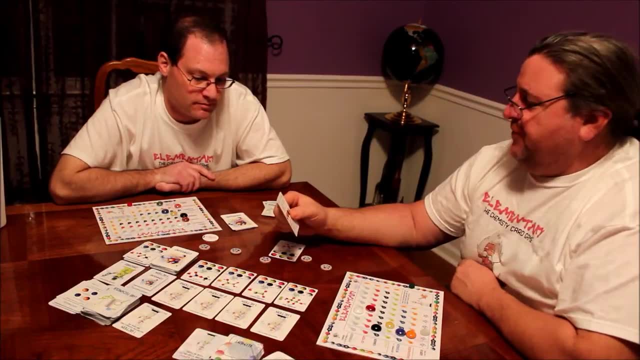 the one action to try to finish this card off- but I'm also going to do- is I'm going to play another lab technique, and this is called disassociate your reaction. It's going to allow me to complete a compound, but without any two common elements. 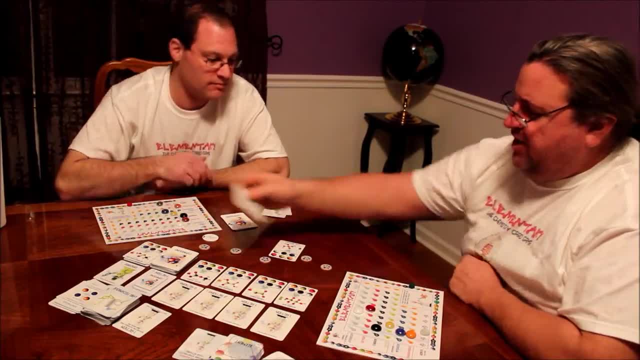 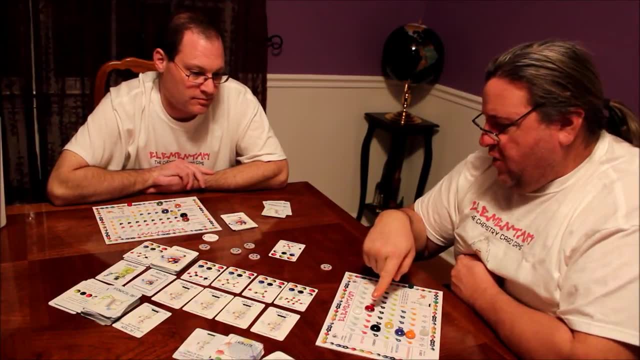 So I can. so two common elements I don't need to do in order to complete it. All right, So that's that. So those are those, that one action and that action. So I will, I will, I will forego, I'll just, I'll just forego hydrogen and oxygen. So I'll just pay one less. So go two down there, pay three oxygen. I'll pay my one phosphorus- I just picked up on the last round- and then I'll spend my two bonds and I will get 10.. 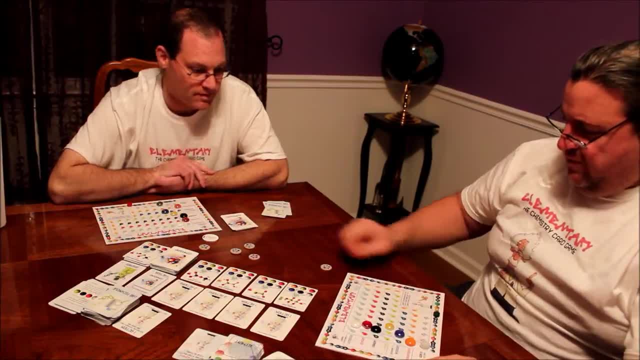 So I'll go from 41,, I'll go away to 51.. All right, So I got one last one action I can. doesn't really do me much of anything, so this is by the box for giggles, and then. 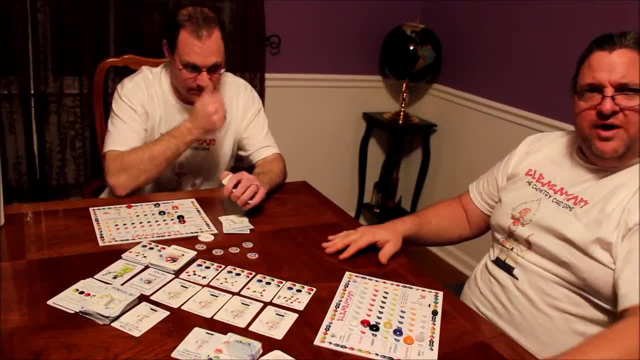 that is now the end of the game. So now we're going to get to end of game scoring and just show you how how that all works out. So Actually it looks like we're both at 51 points. Yep. 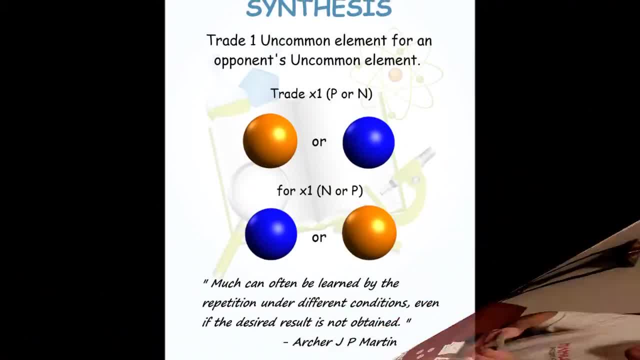 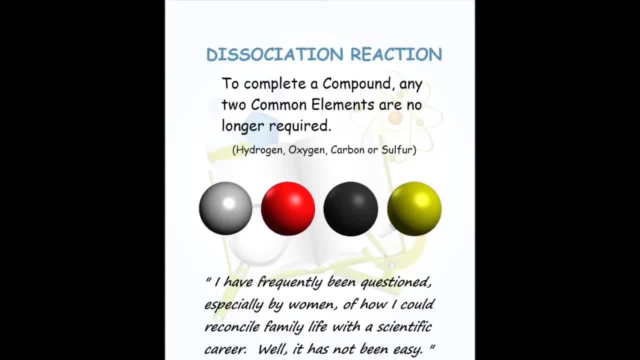 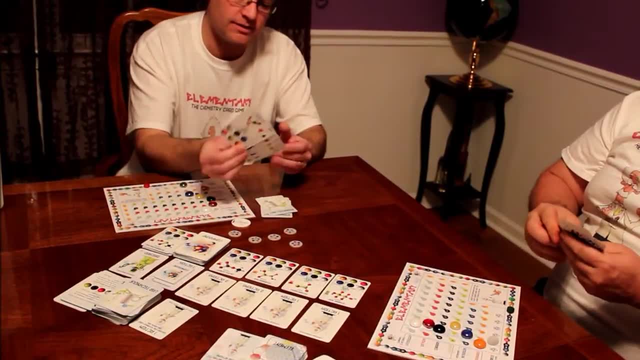 Yep, Yep, Yep, Yep, Yep. Okay, so I went first, so I will show what I had first here. All right, so I was able to collect a complete set of one of each card, one of each lab glassware.